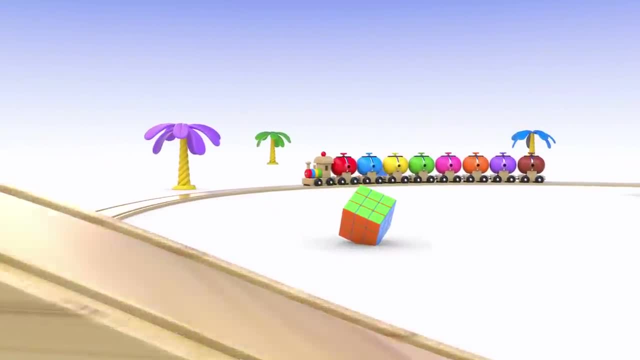 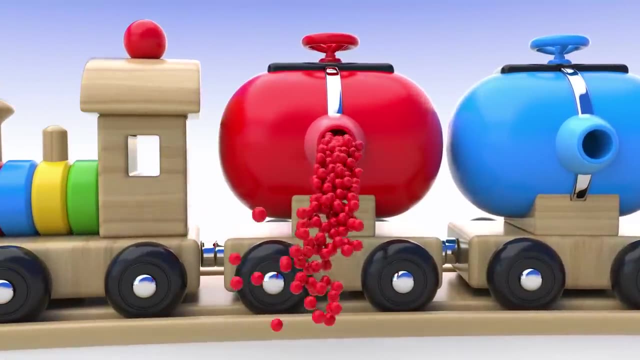 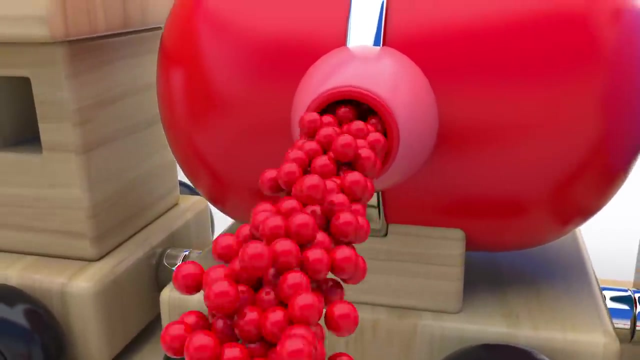 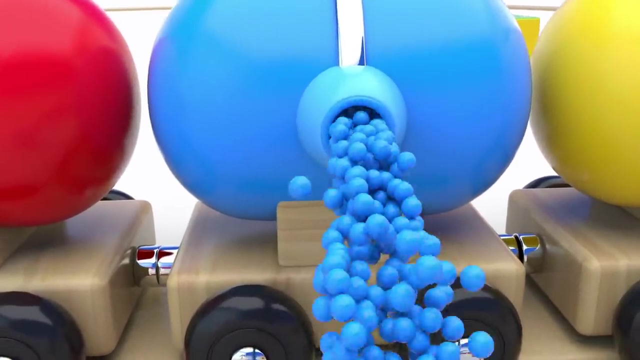 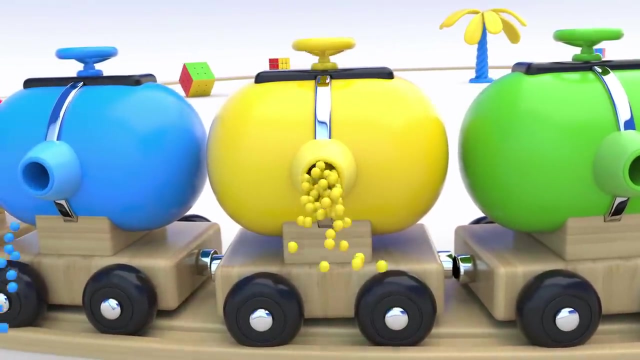 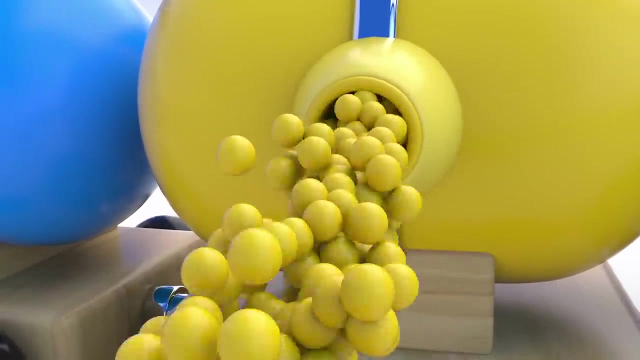 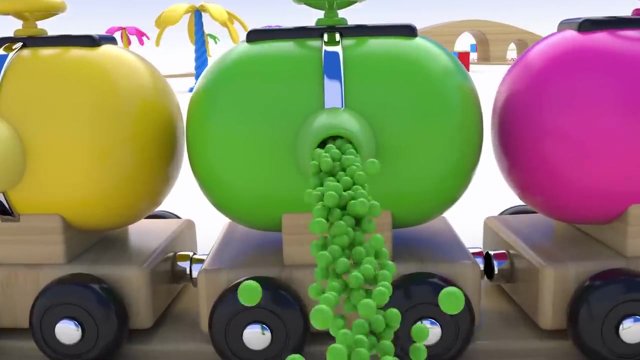 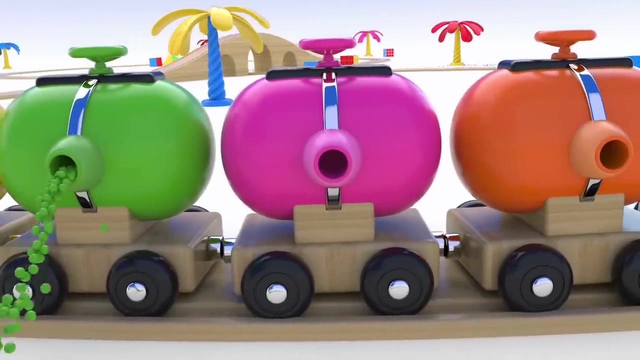 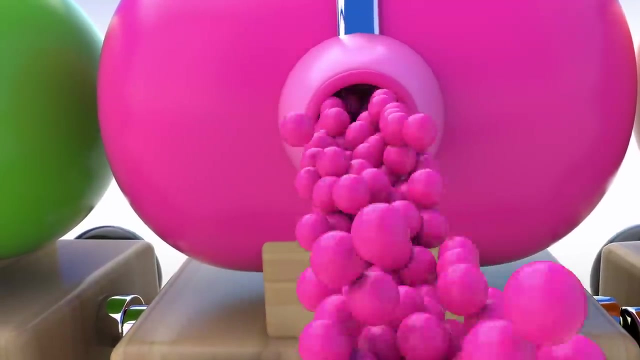 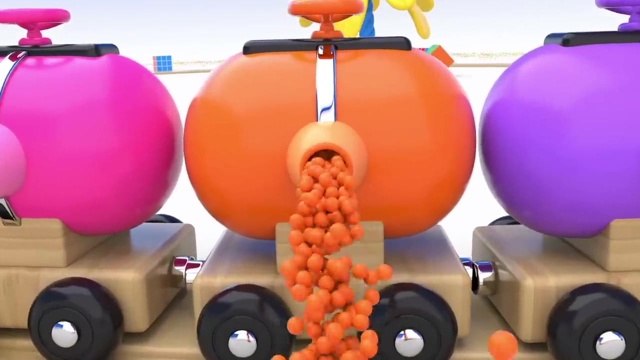 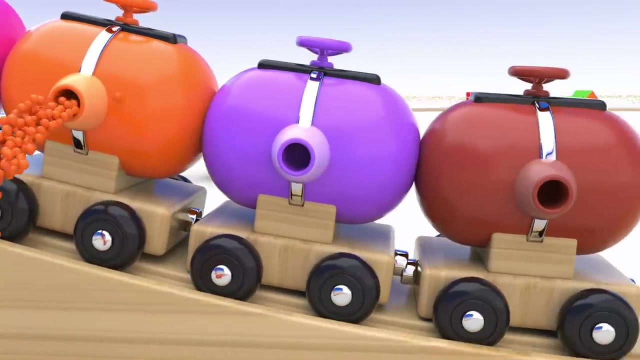 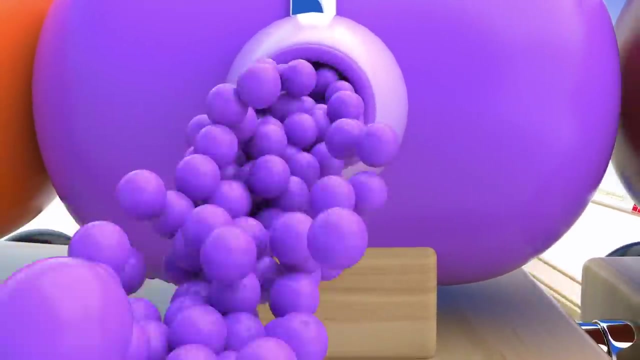 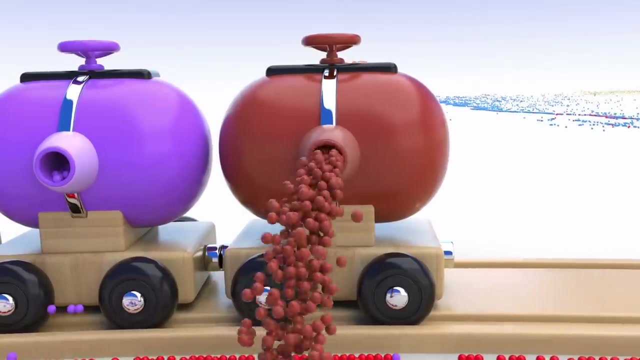 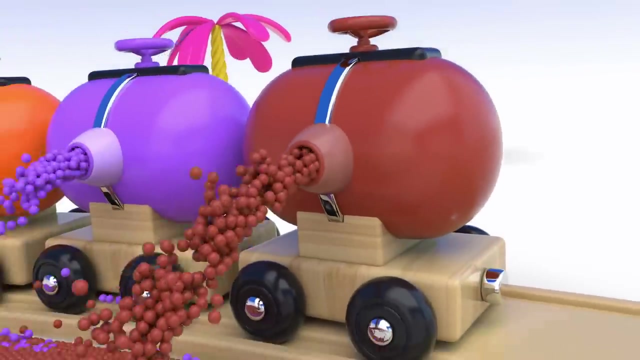 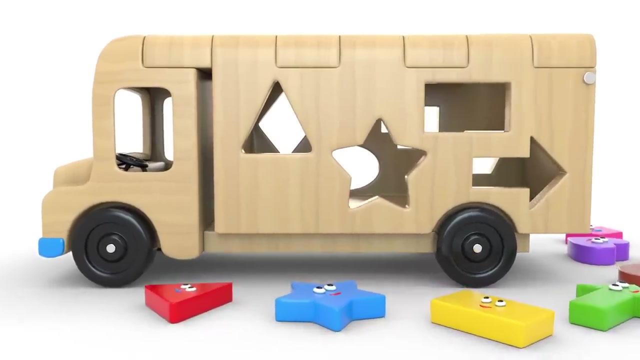 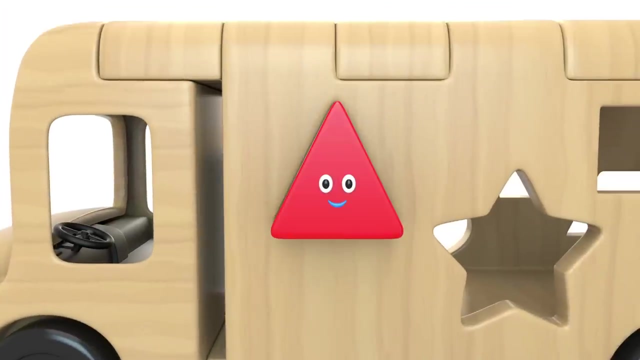 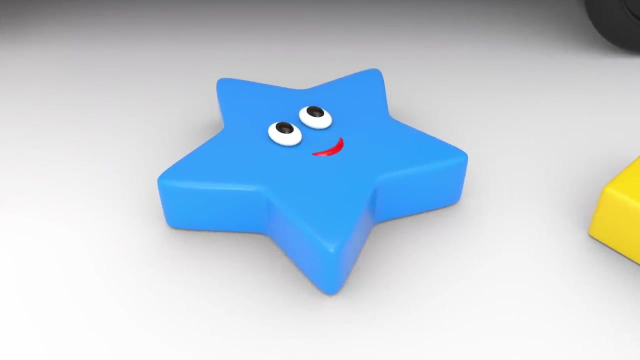 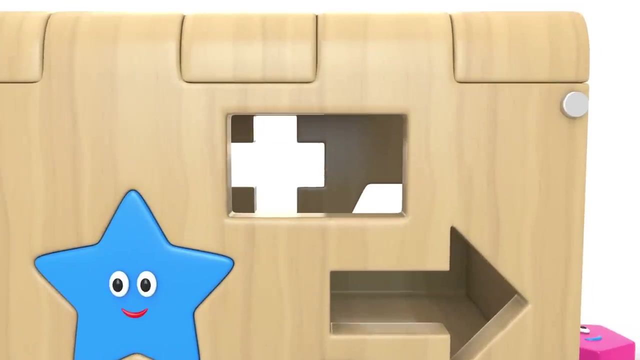 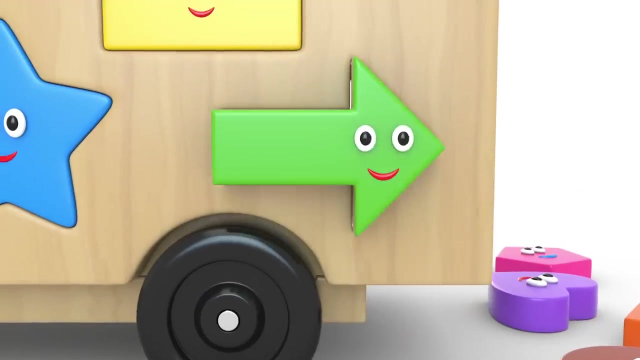 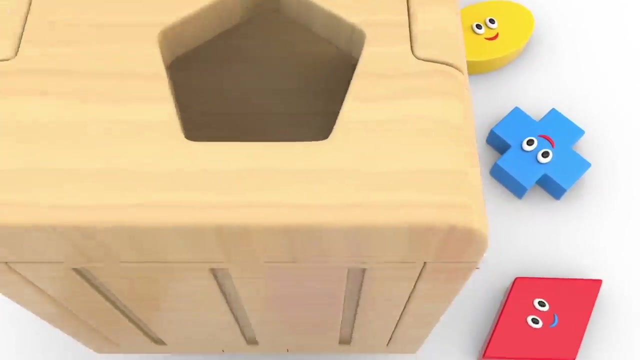 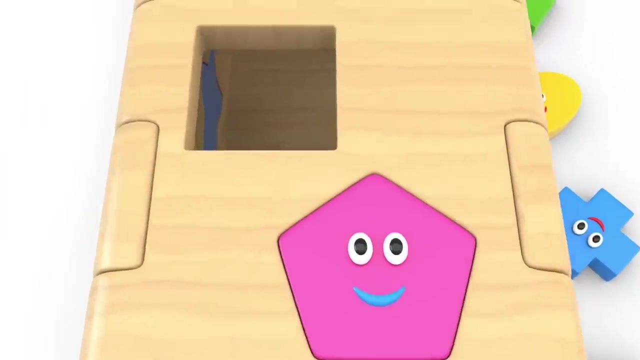 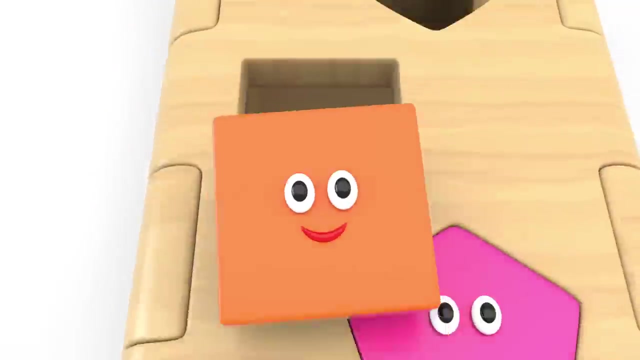 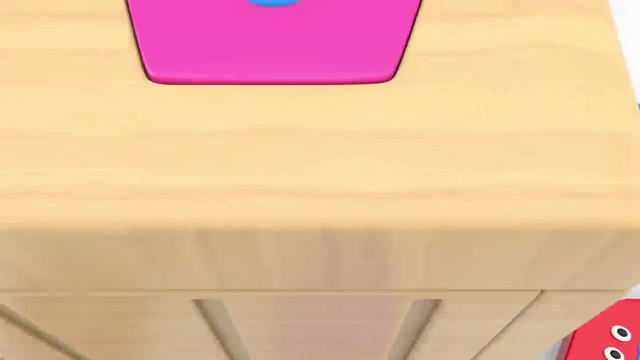 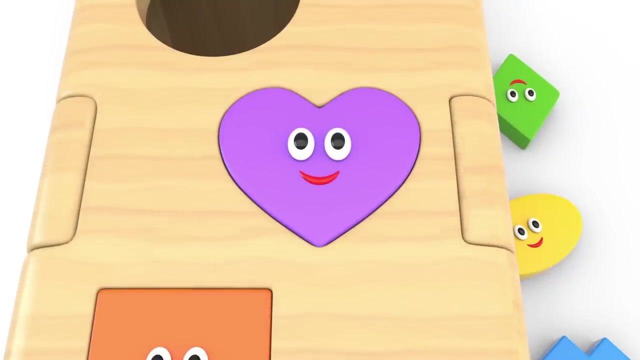 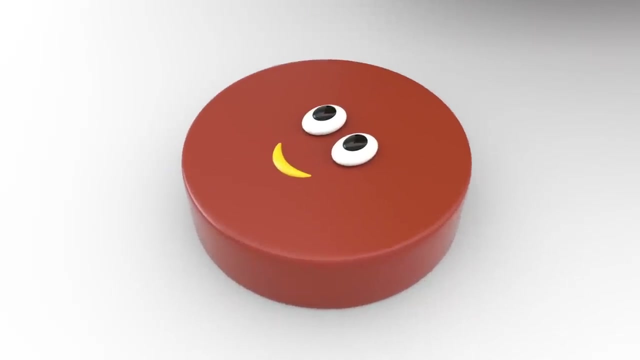 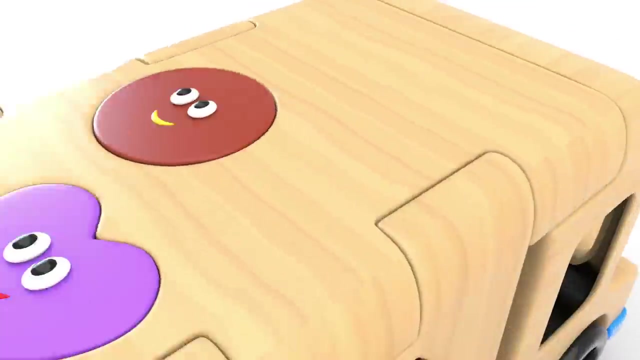 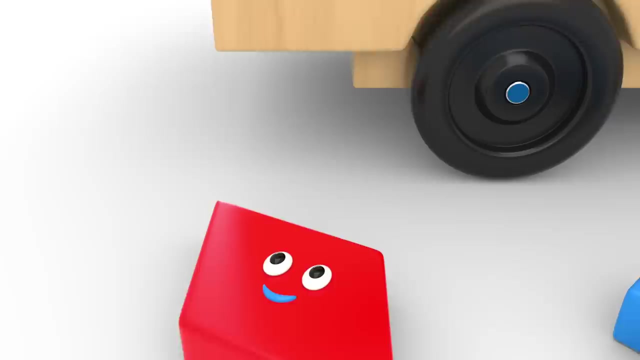 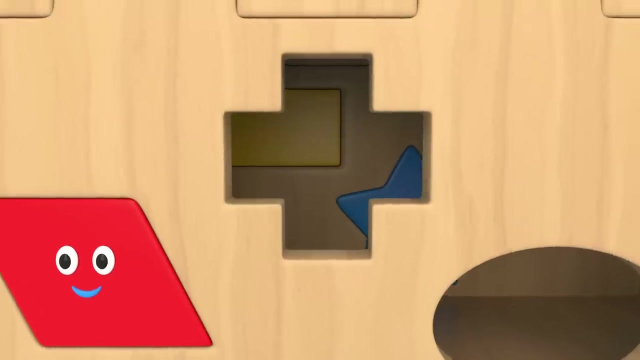 Please add punctuation in the appropriate places: yellow, yellow, green, green, pink, pink, pink, orange, orange, purple, purple, brown, brown. Wow, That's fantastic. triangle, triangle, star, star, star, star, rectangle, rectangle, rectangle, rectangle, rectangle, arrow, arrow. pentagon, pentagon, pentagon, square, heart, circle, circle, parallelogram. 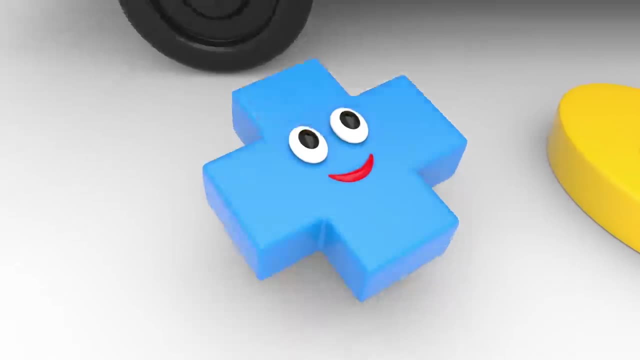 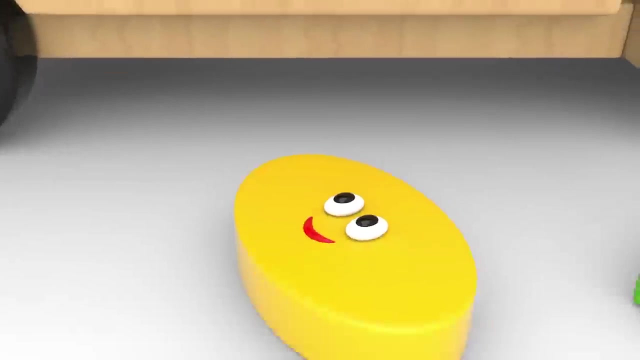 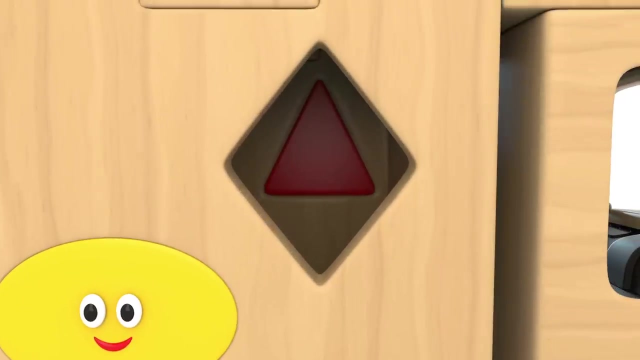 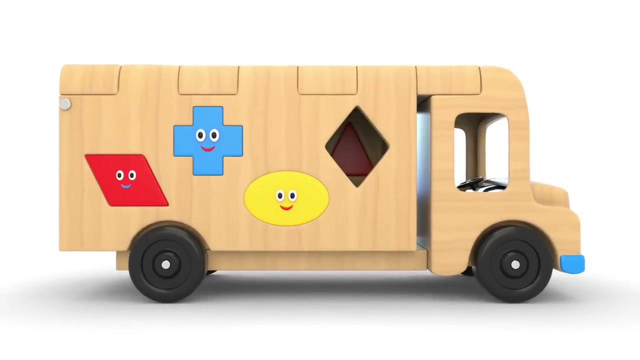 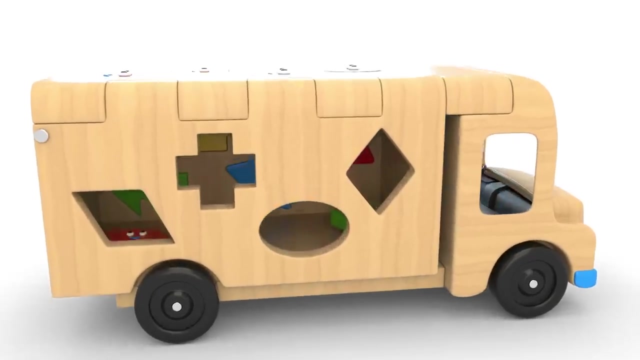 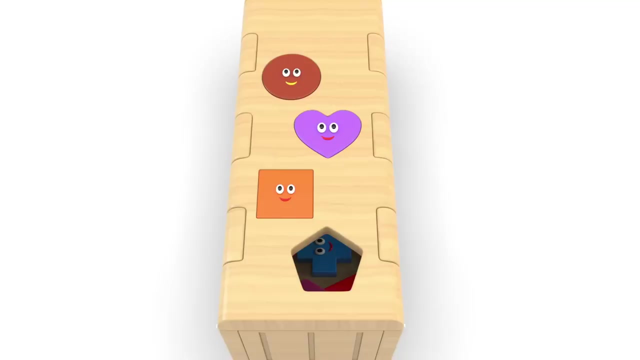 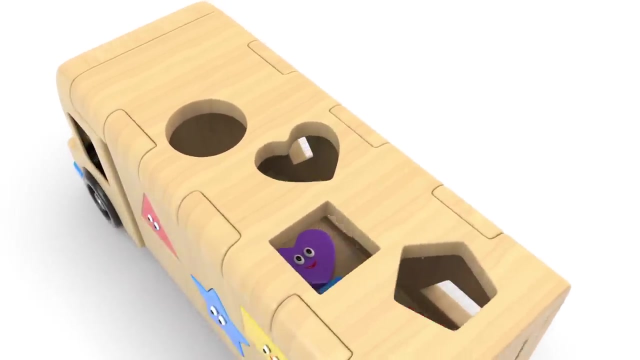 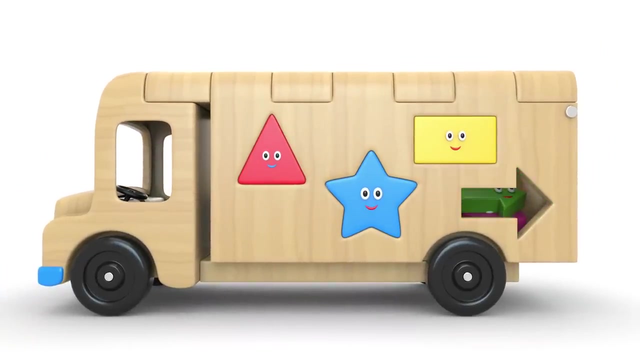 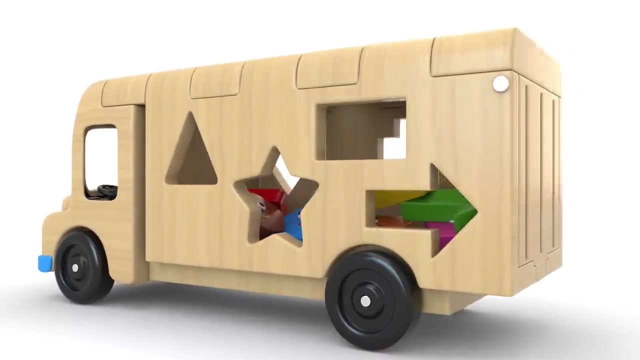 cross parallelogram: oval, oval rhombus, rhombus, rhombus, oval, cross parallelogram- pentagon, pentagon, pentagon, square, square, heart, heart circle, circle, arrow, arrow, rectangle, rectangle, star, star triangle, triangle, triangle triangle, spiral window line 10, 10, 8. 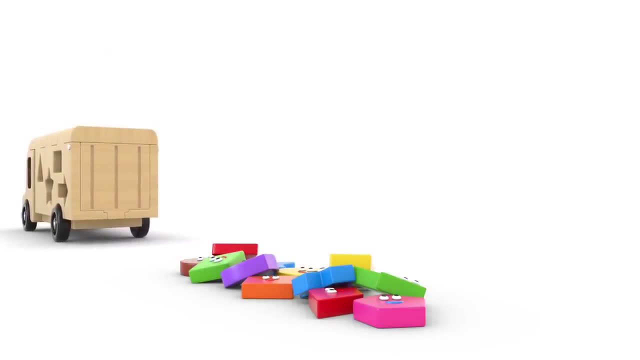 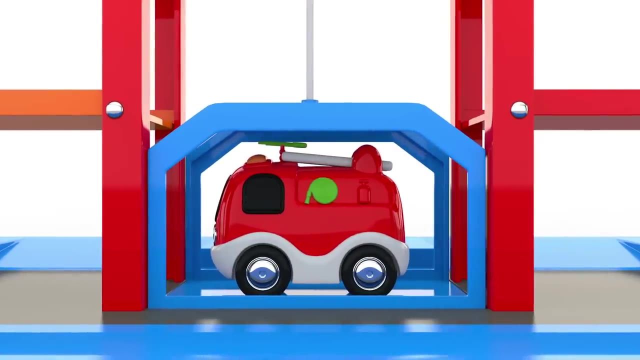 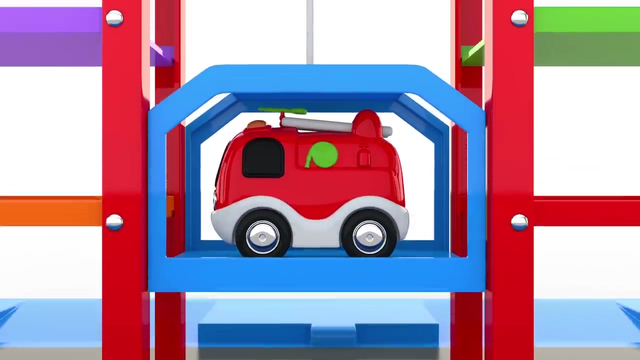 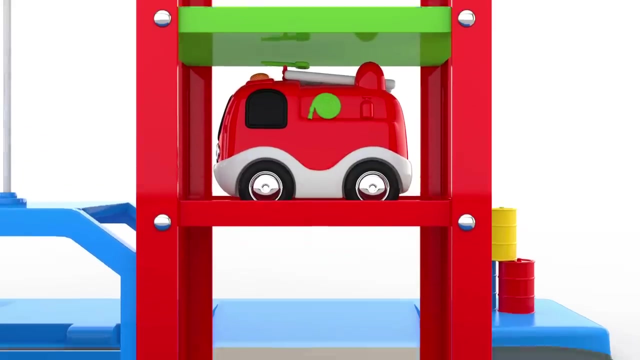 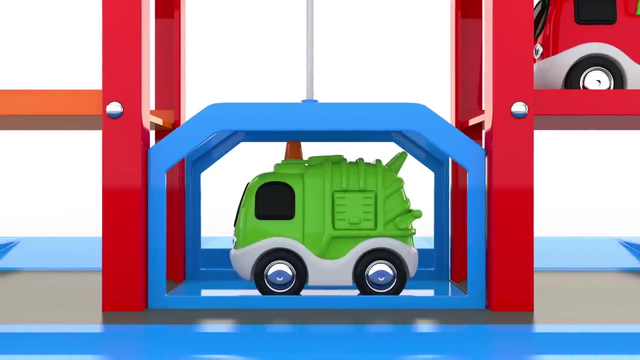 8, 7, 9, 10, 11, 11, 12, 12, 13, 14, 15, 16, 17, 18, 19, 20, 21, 23, 24, 23, 24, 25, 26, 26 Green garbage truck. 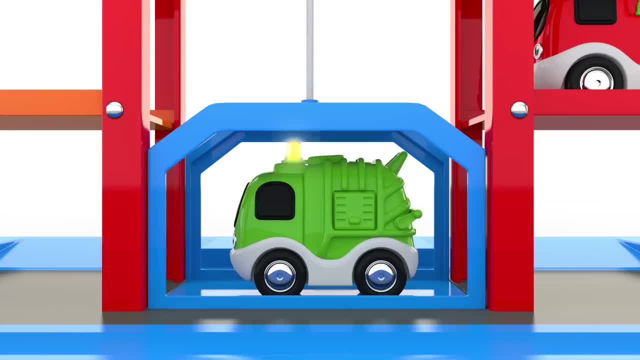 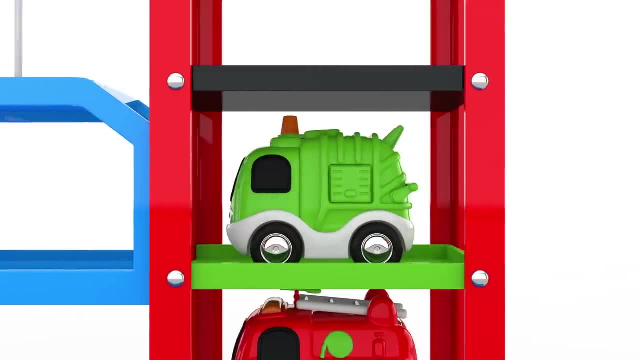 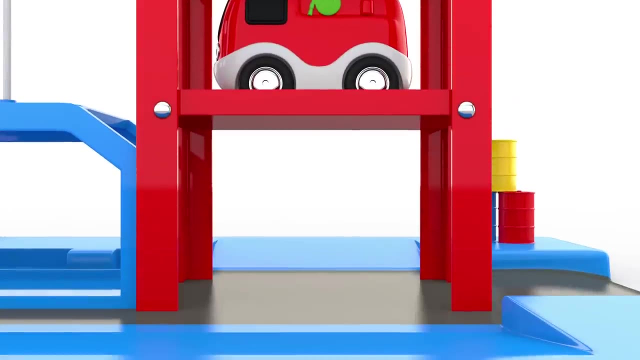 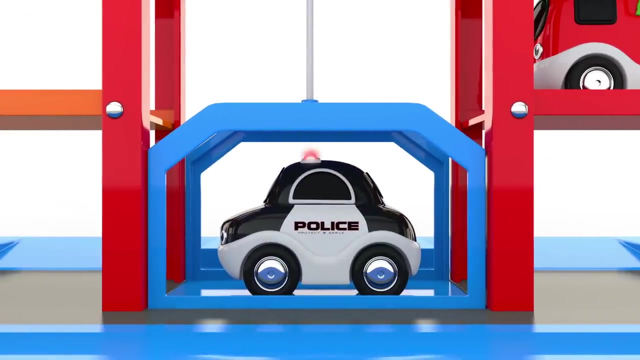 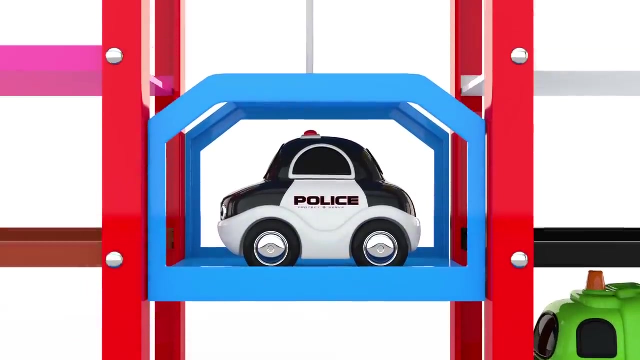 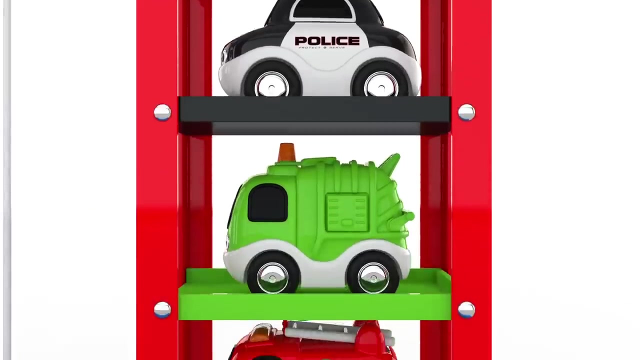 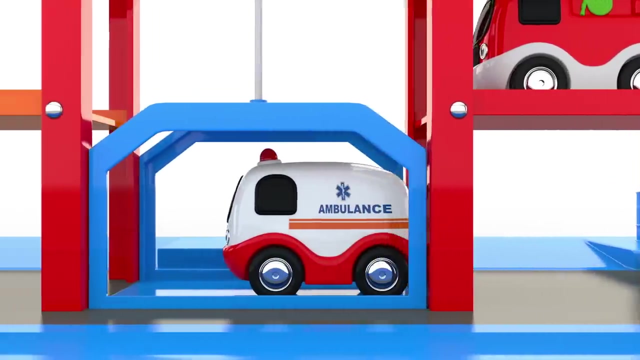 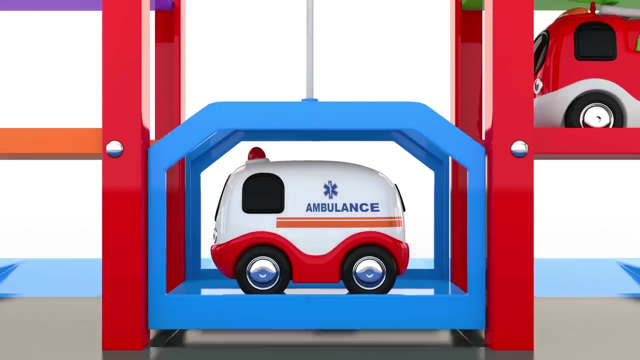 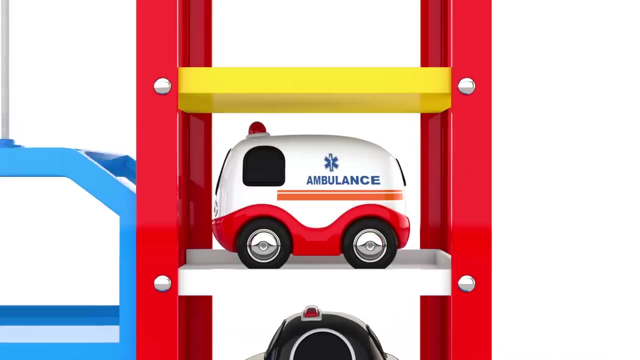 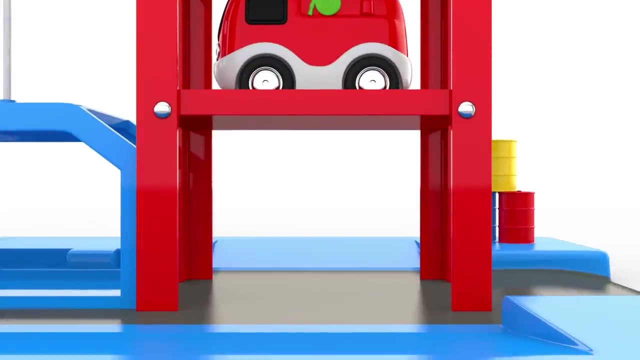 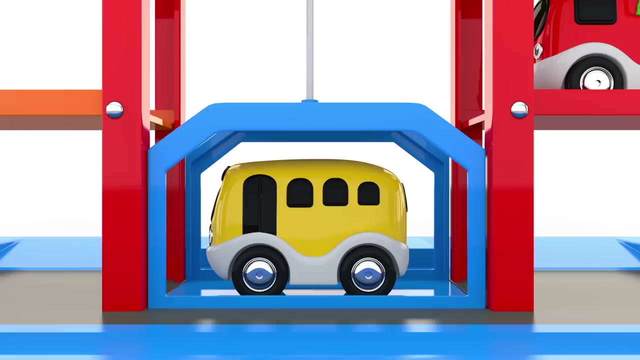 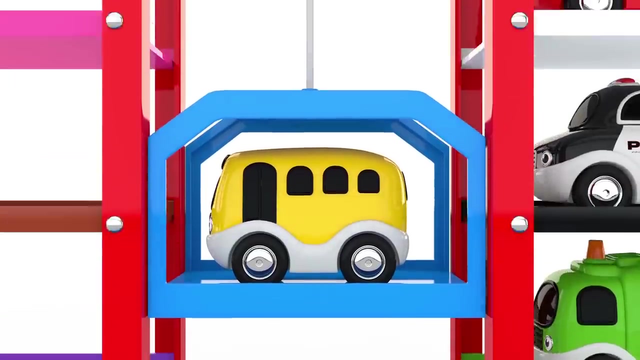 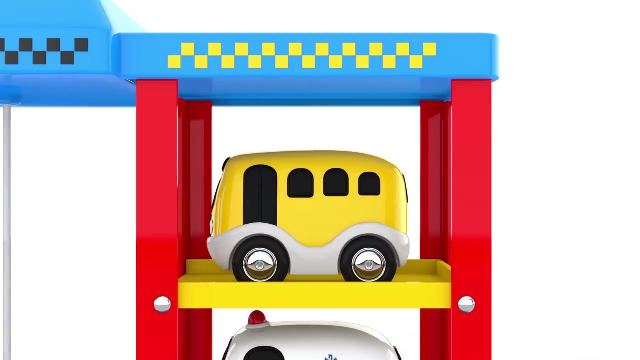 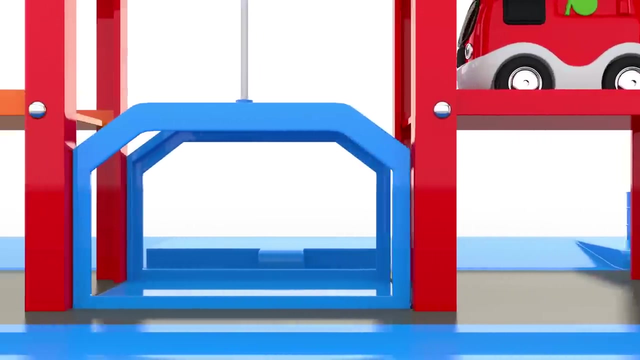 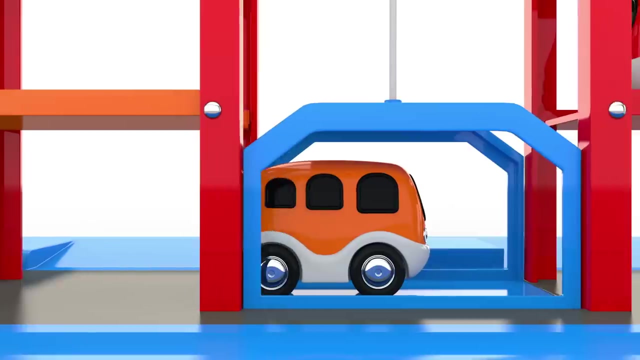 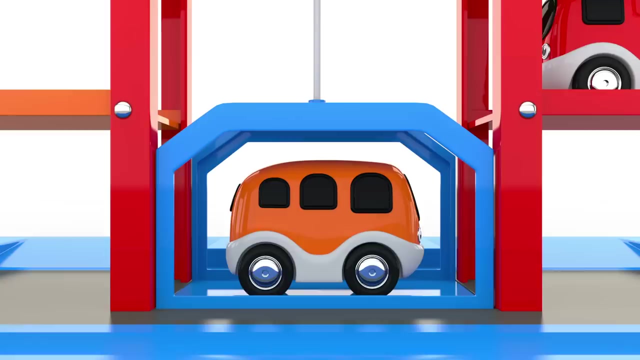 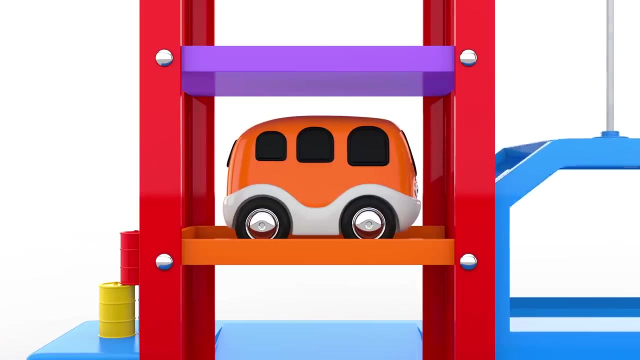 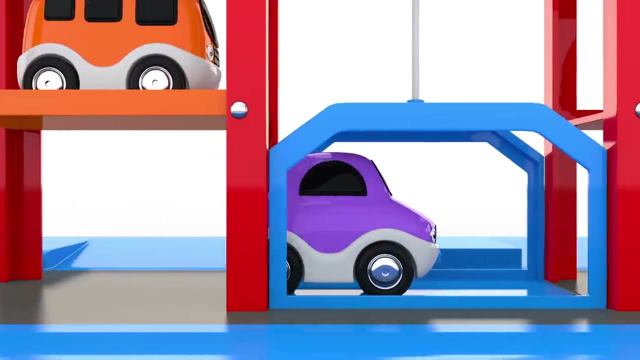 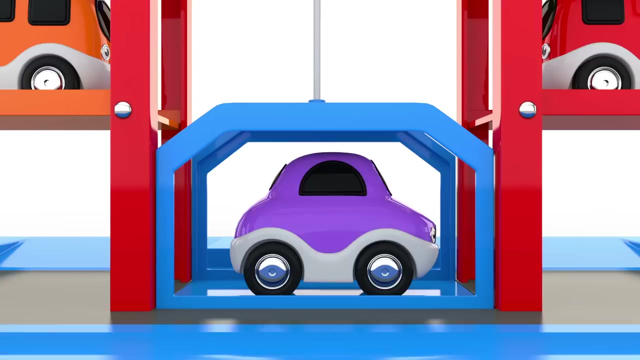 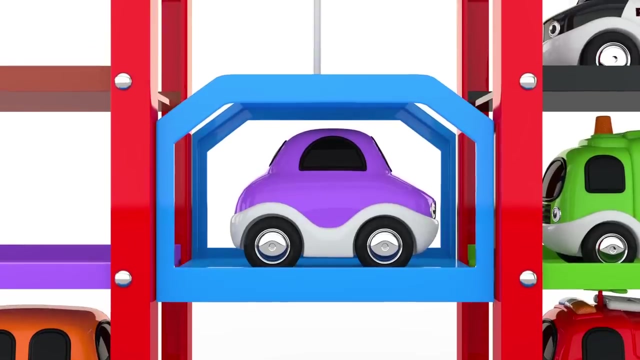 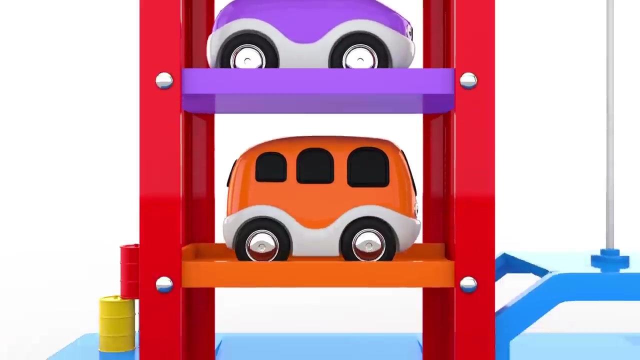 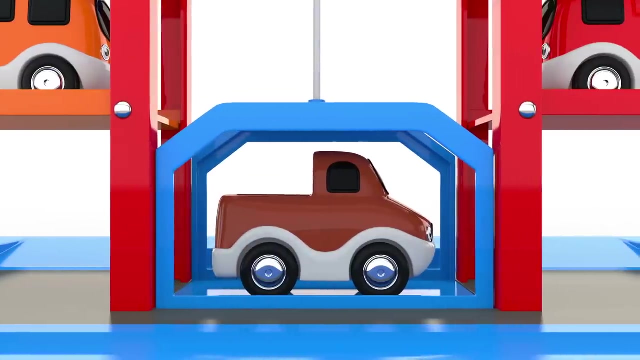 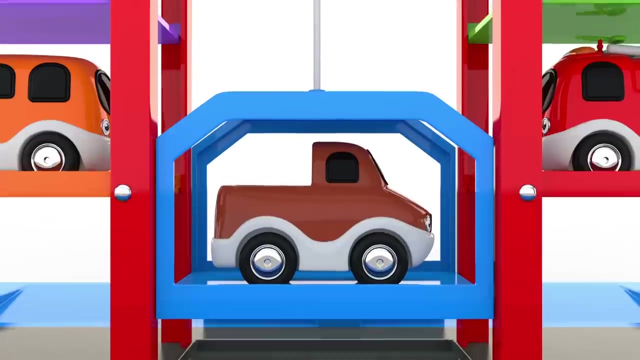 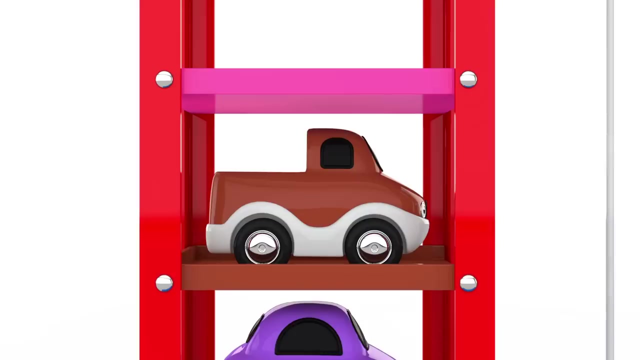 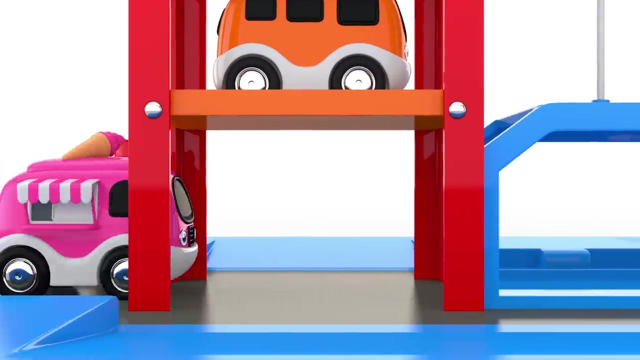 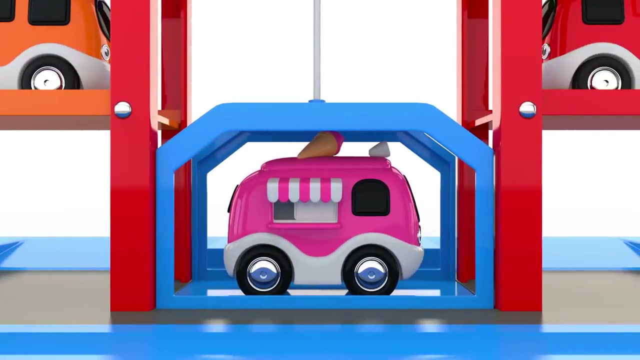 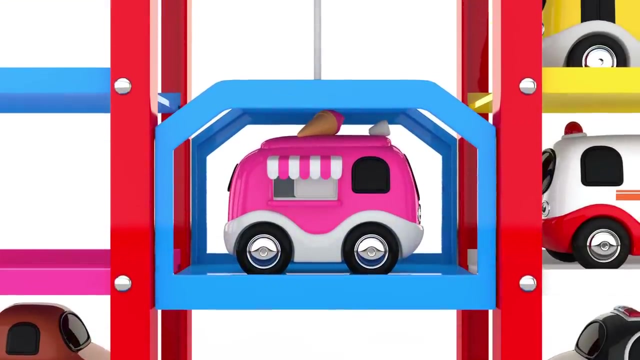 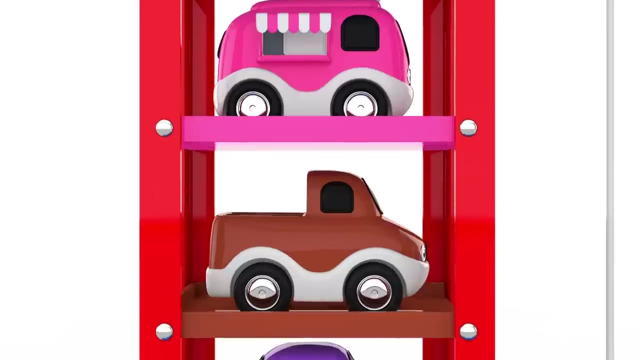 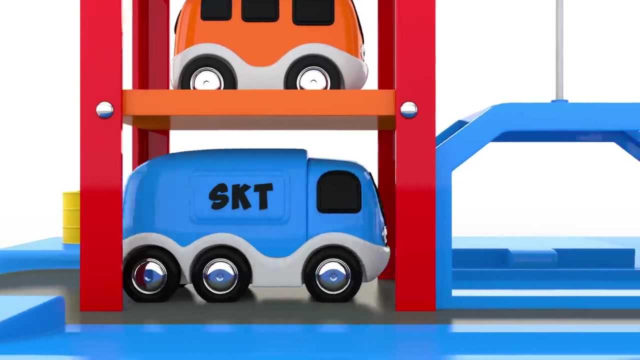 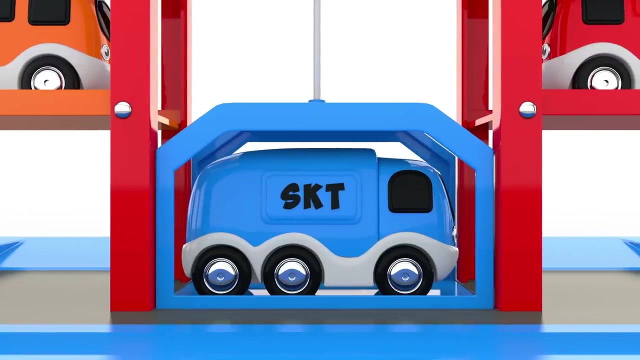 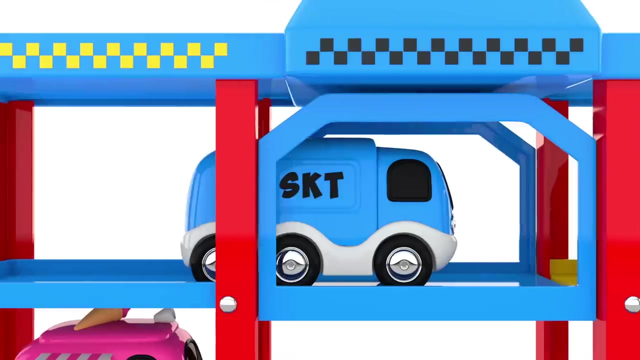 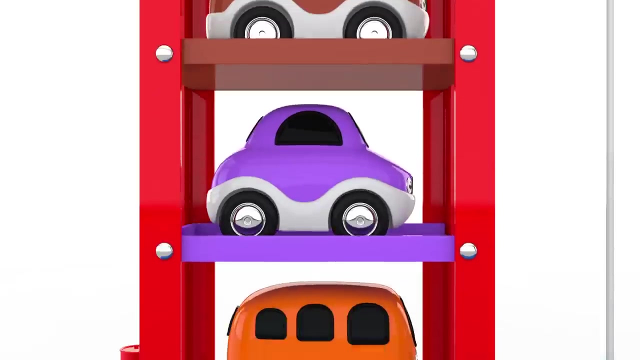 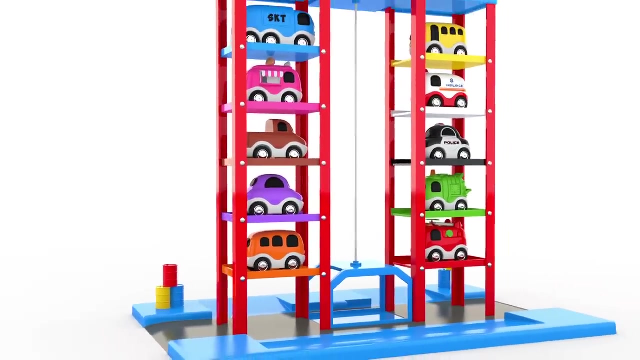 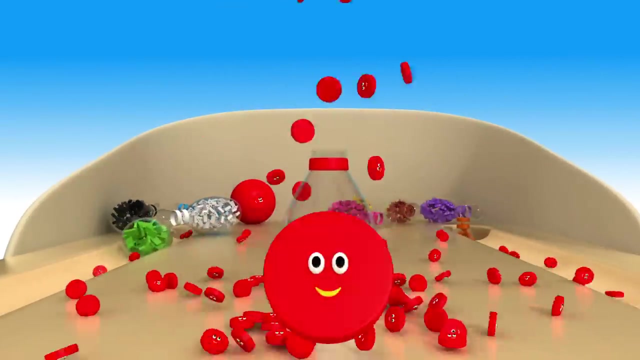 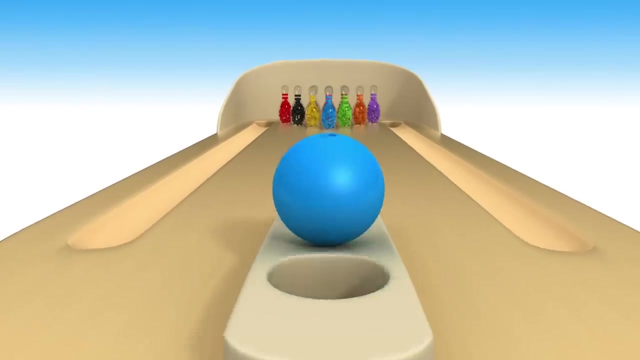 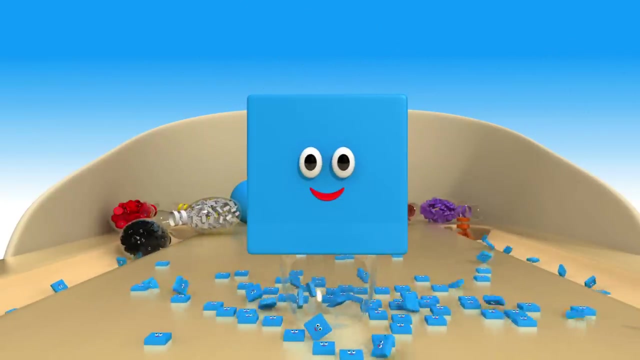 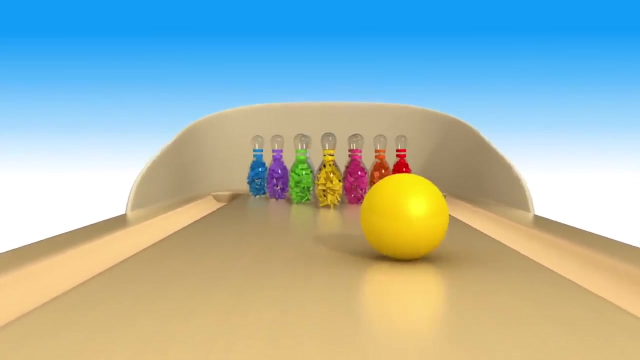 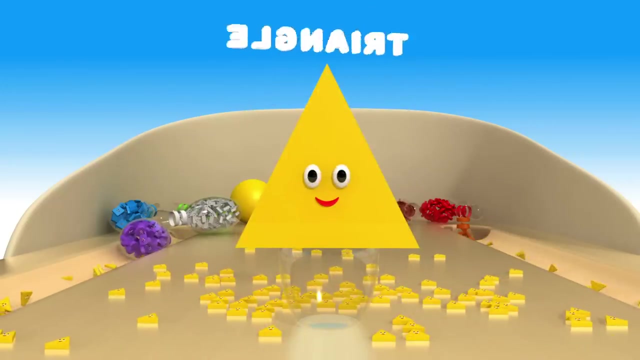 Green Black police car. Black White ambulance. White Yellow school bus. Yellow White bus. Yellow school bus. Yellow school bus. Yellow school bus. Orange van Orange. Purple car. Purple car. Brown pickup truck. Brown pickup truck. brown pink ice cream truck. pink blue truck. blue red circle. blue square. yellow triangle. 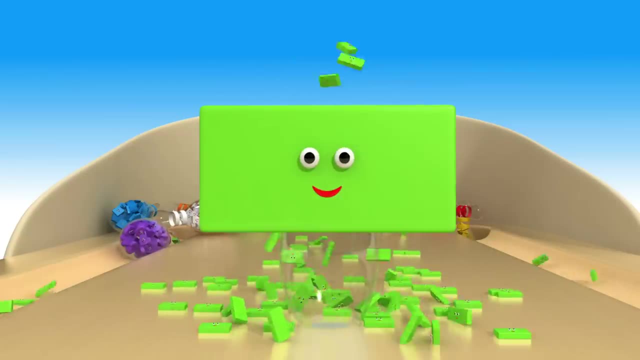 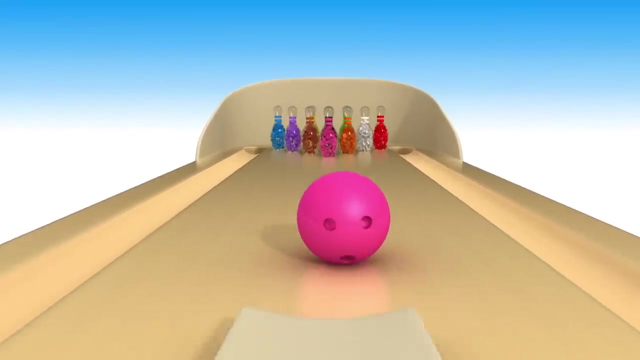 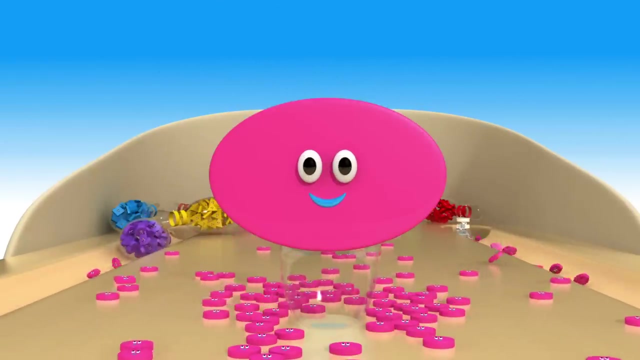 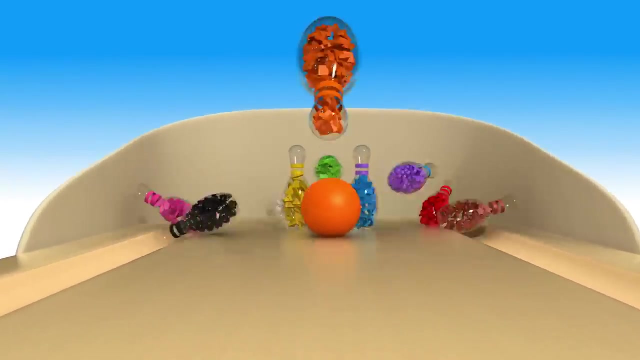 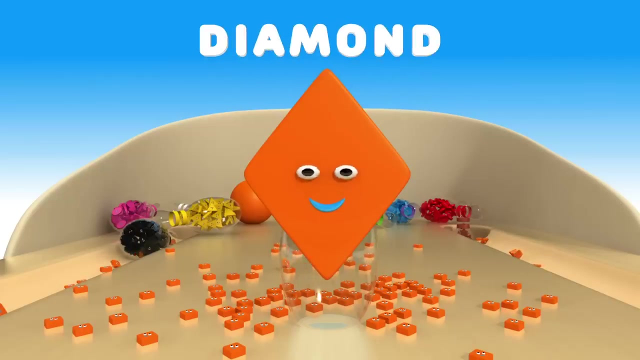 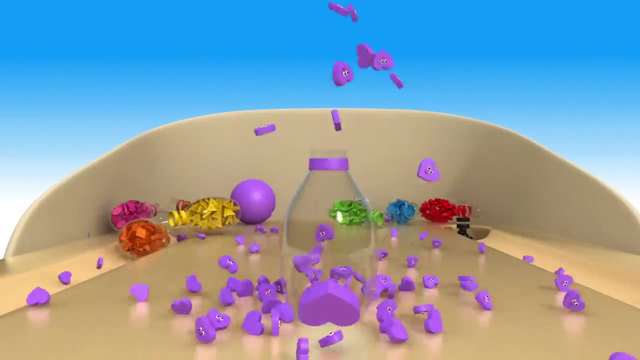 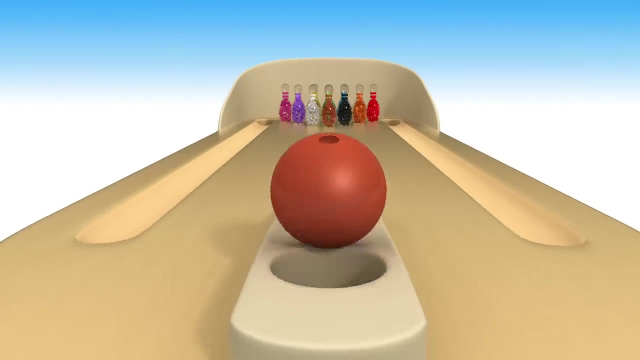 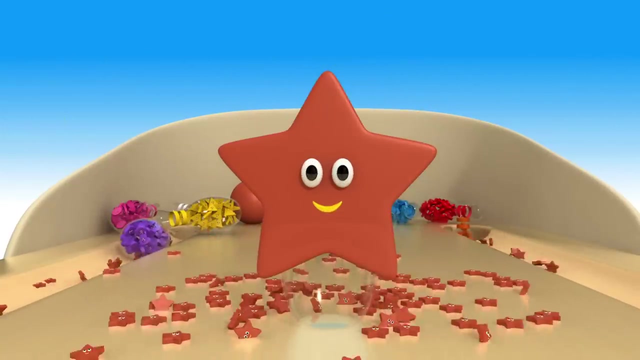 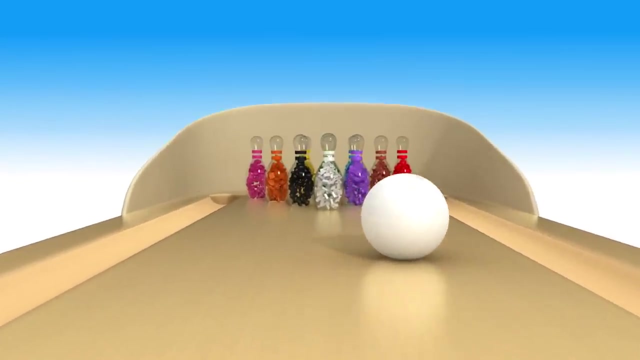 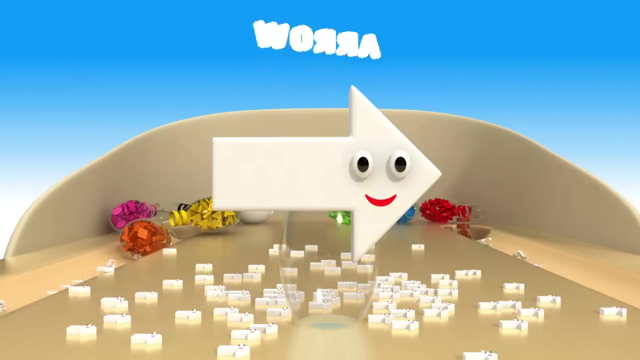 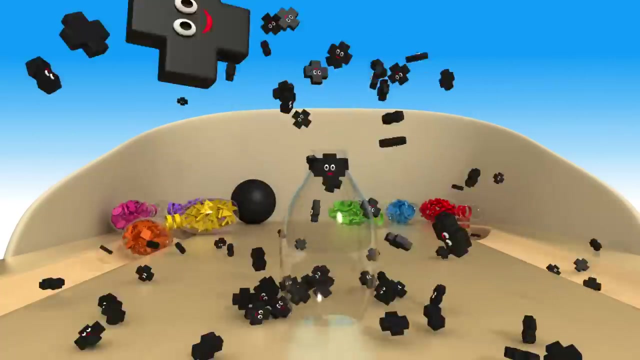 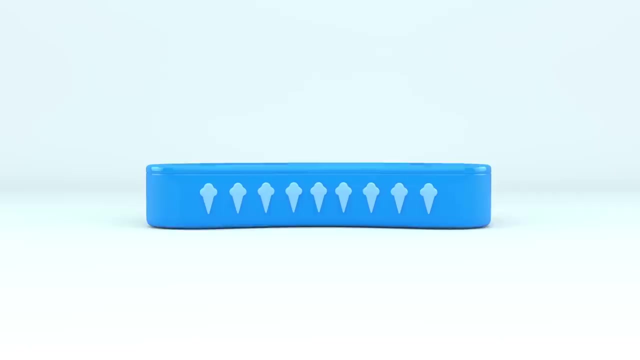 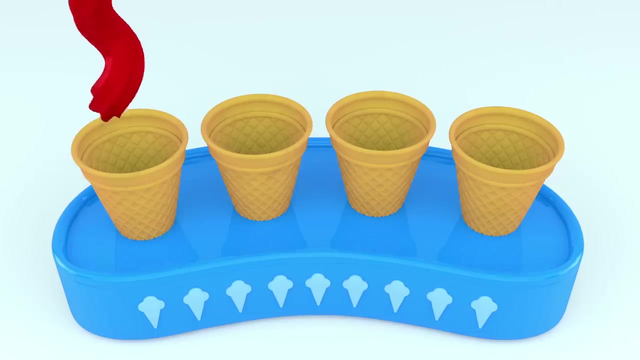 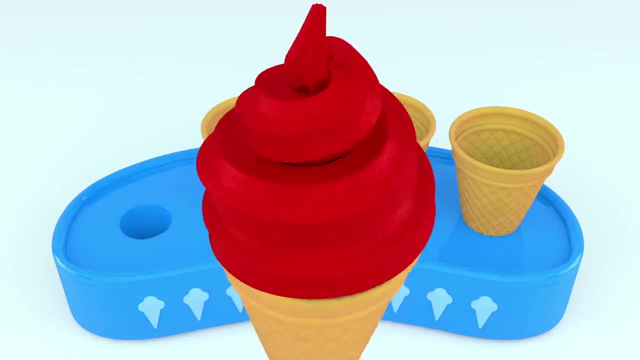 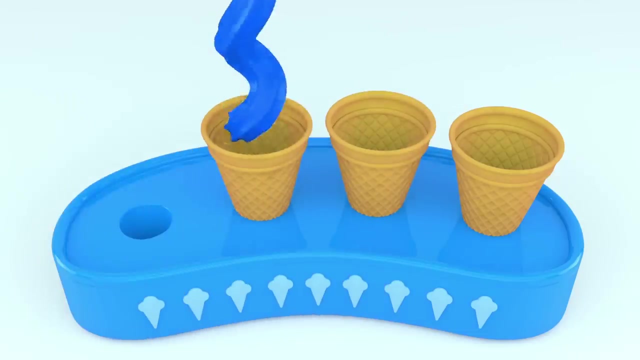 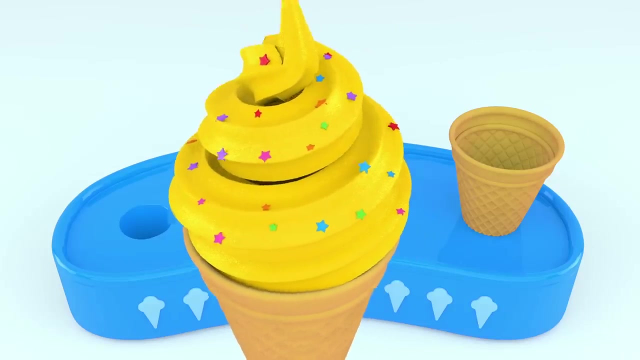 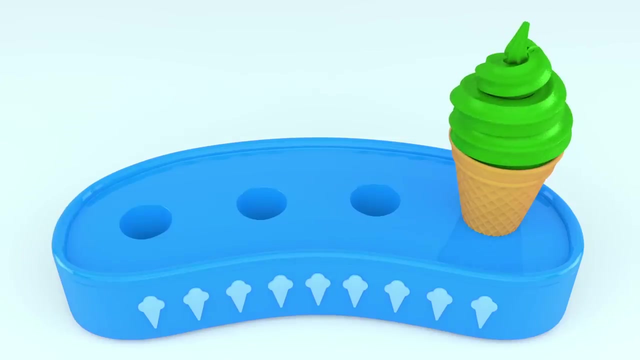 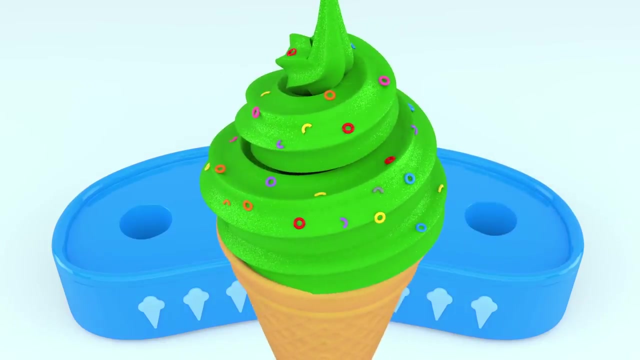 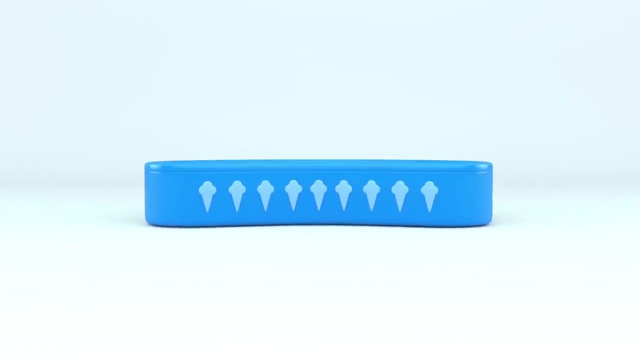 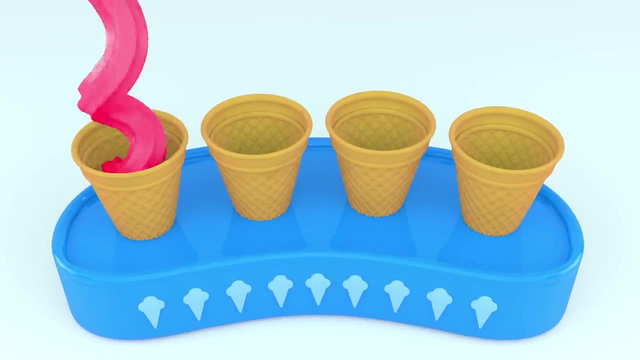 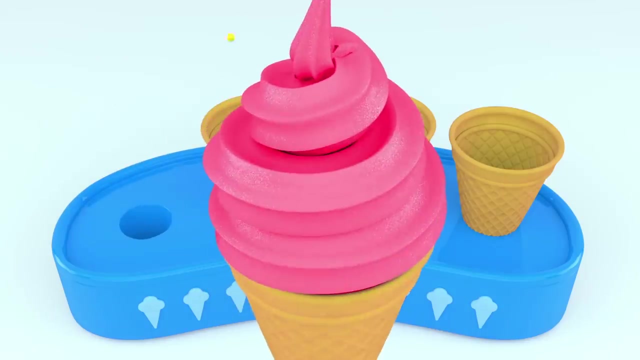 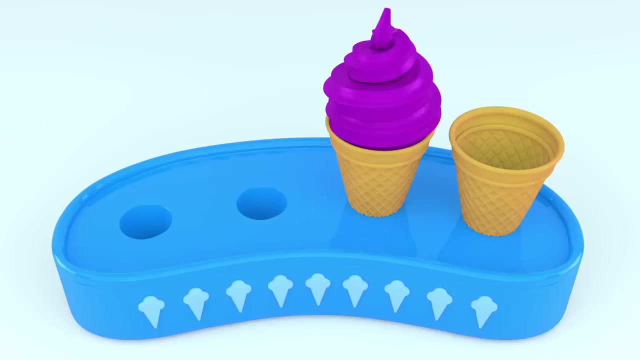 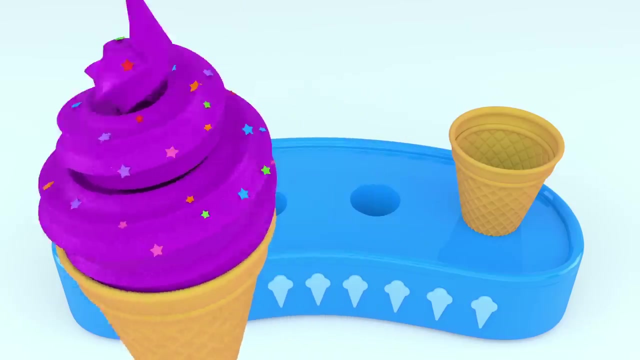 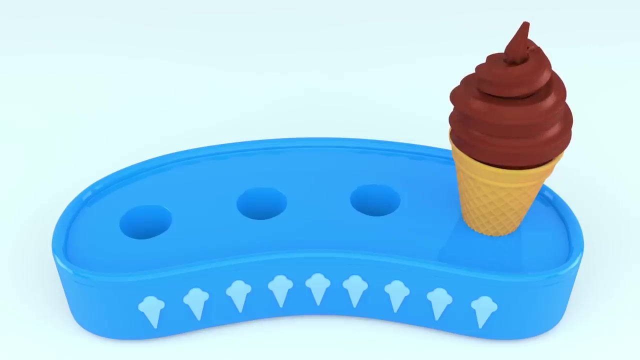 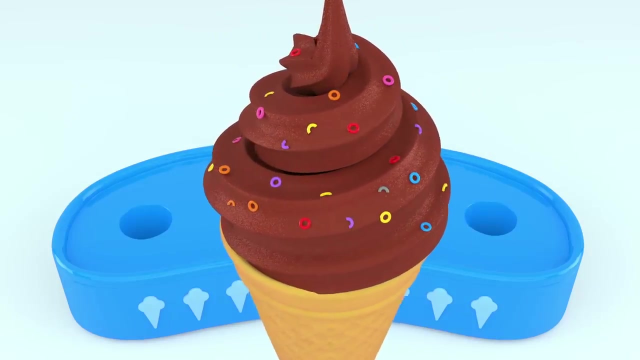 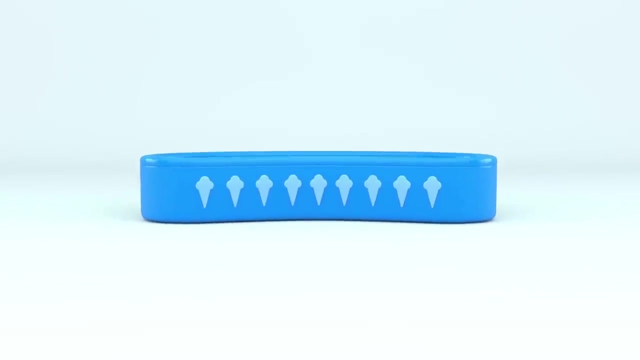 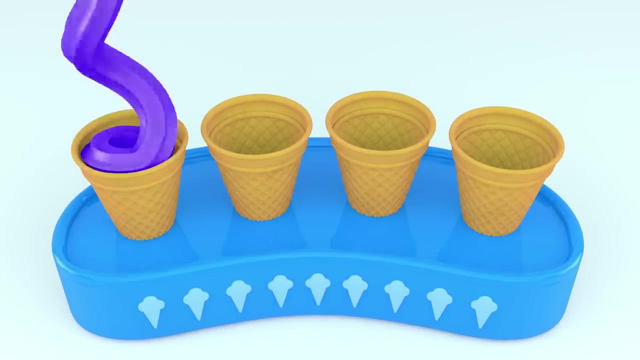 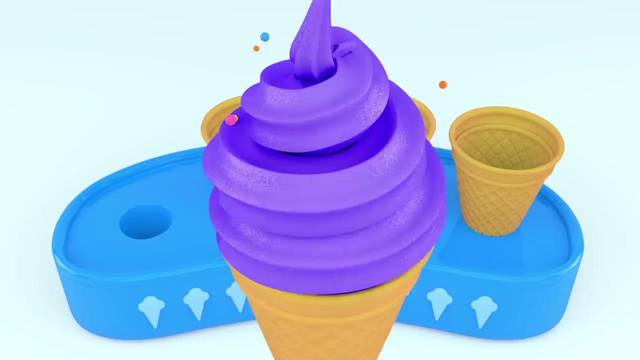 green rectangle, pink, oval, orange, diamond, purple, purple, heart, brown star, white, blue, arrow, black, blue, cross, red, red, red, blue, blue, blue, blue, yellow, yellow, yellow, yellow, yellow, green, yellow, yellow, yellow, green, green, green, green, yellow, green, pink, pink, orange, orange, purple, purple, brown, brown, brown, violet, violet, violet. 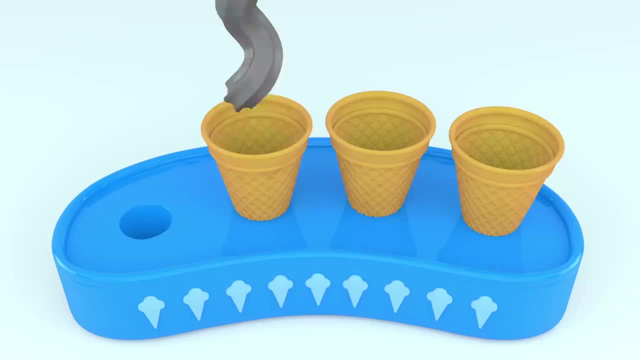 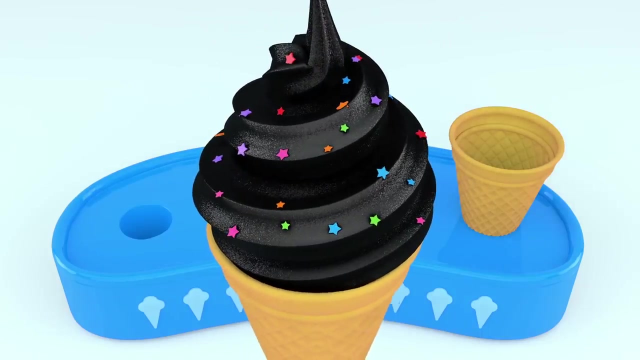 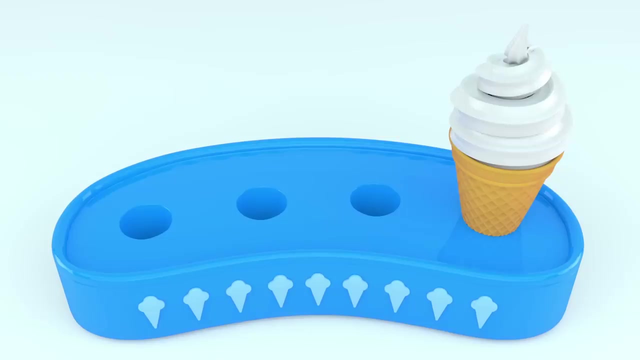 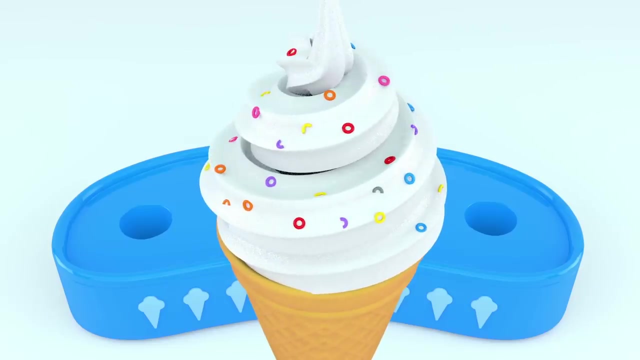 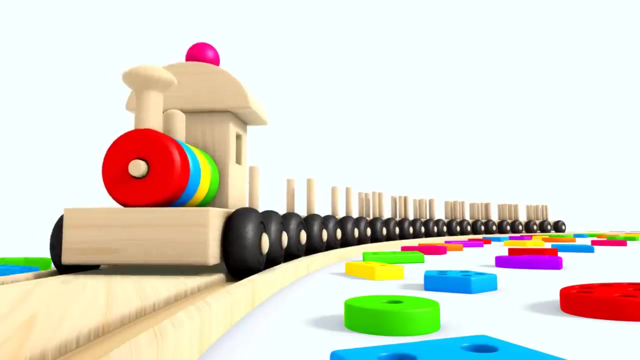 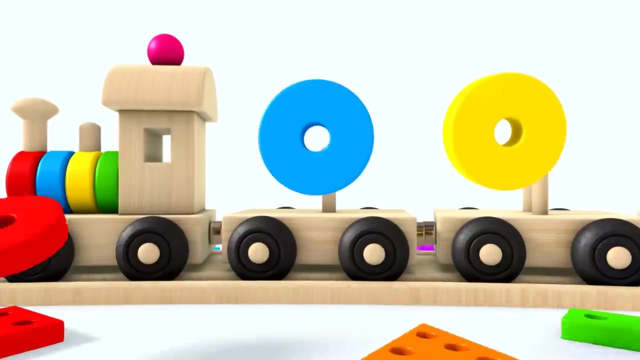 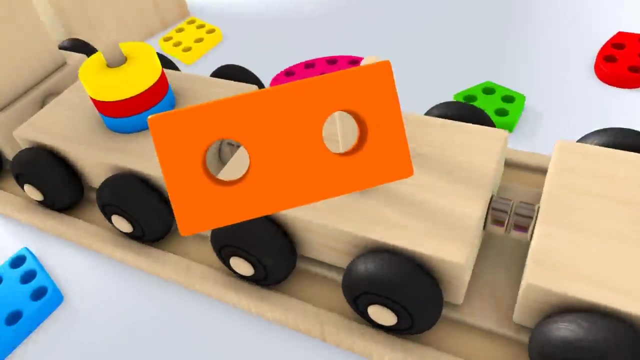 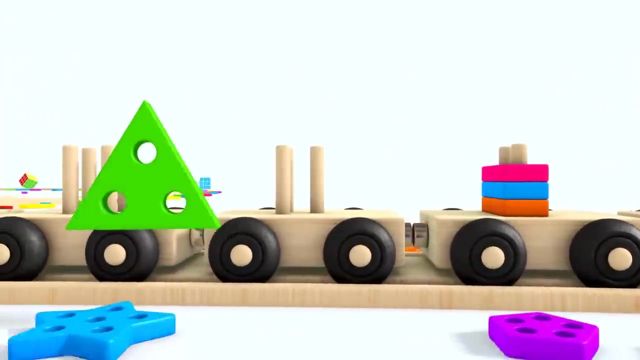 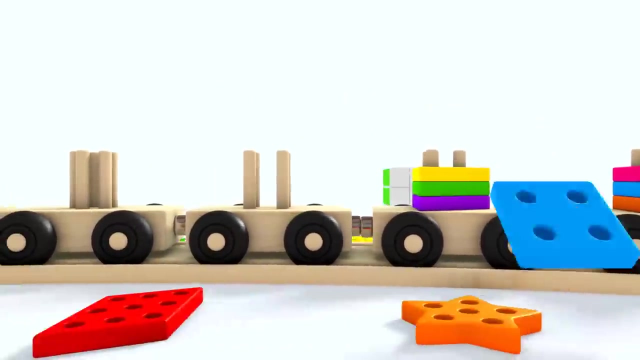 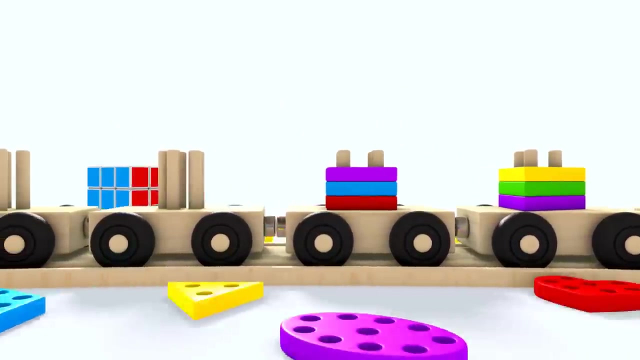 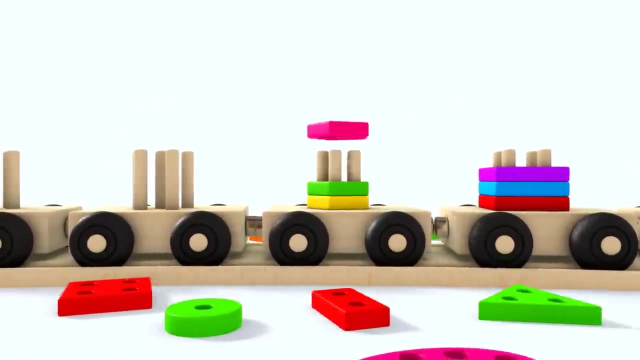 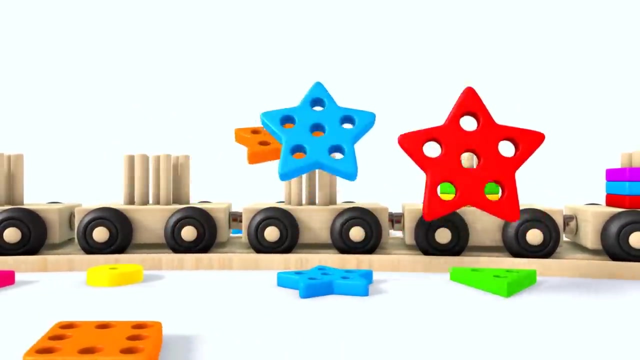 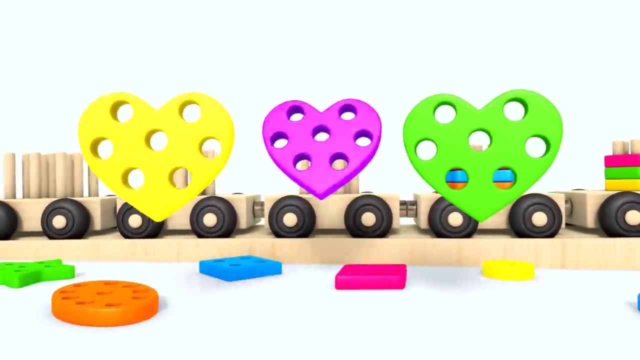 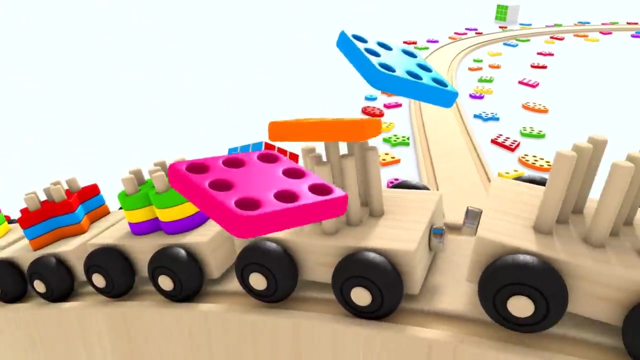 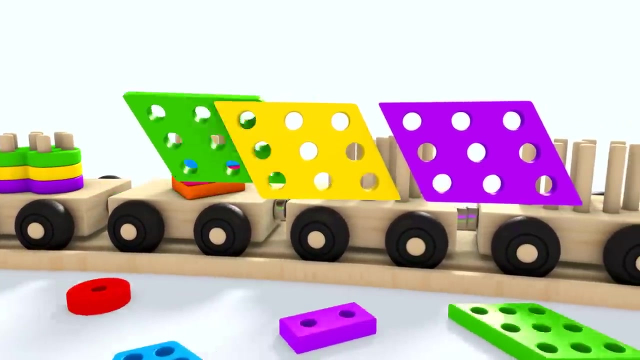 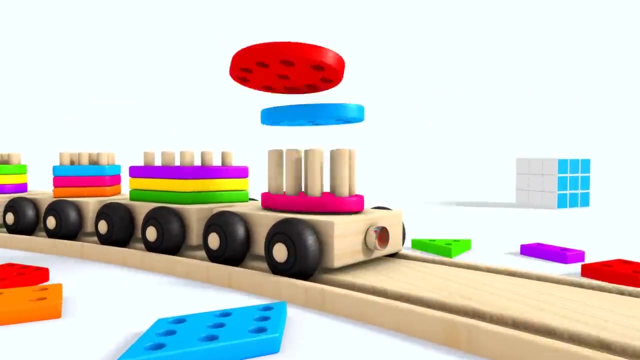 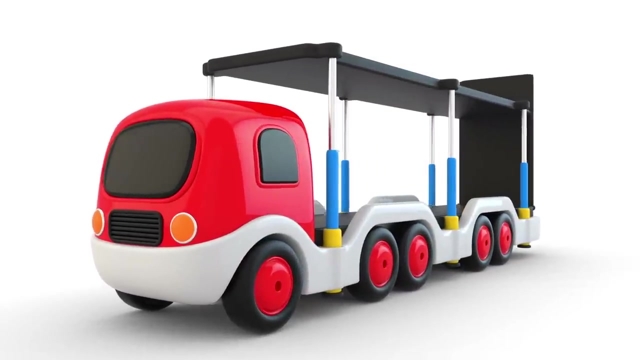 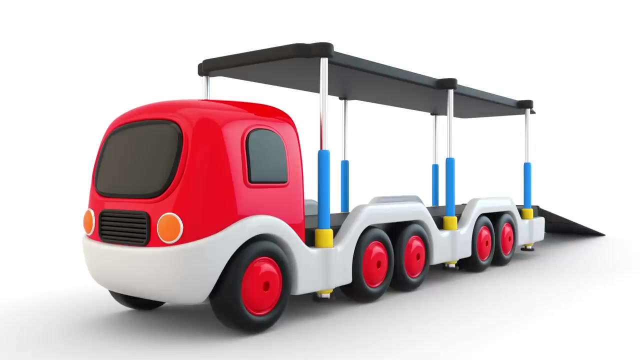 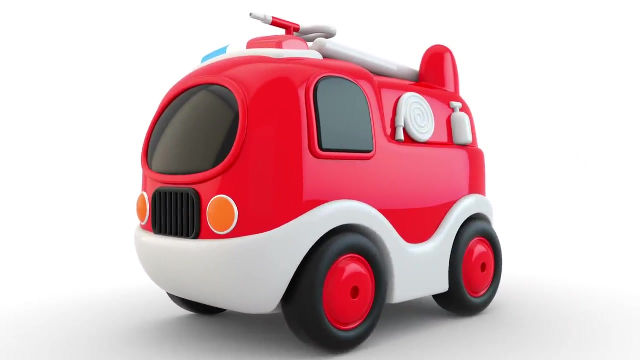 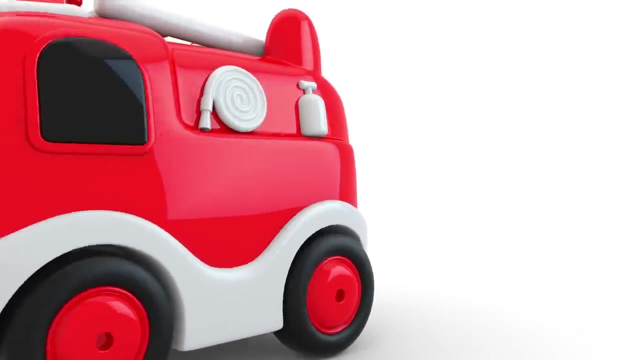 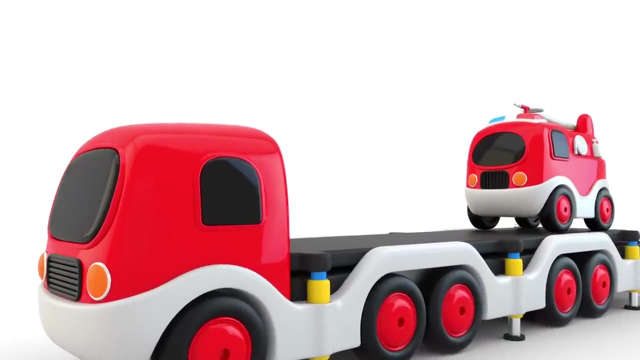 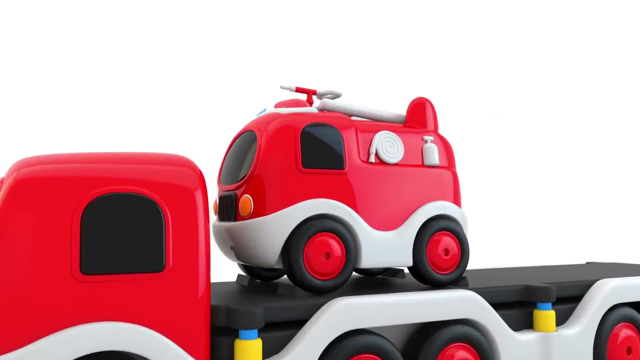 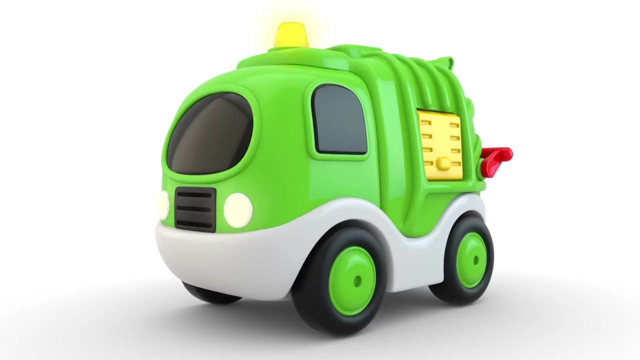 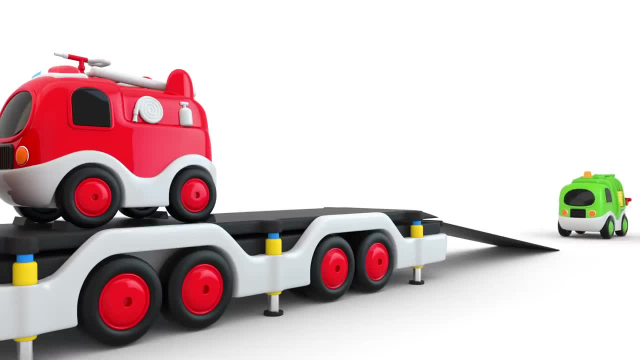 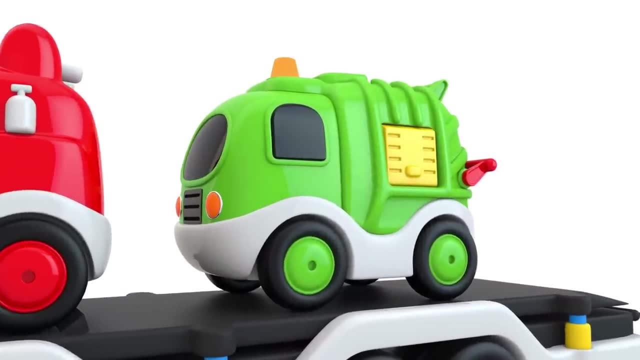 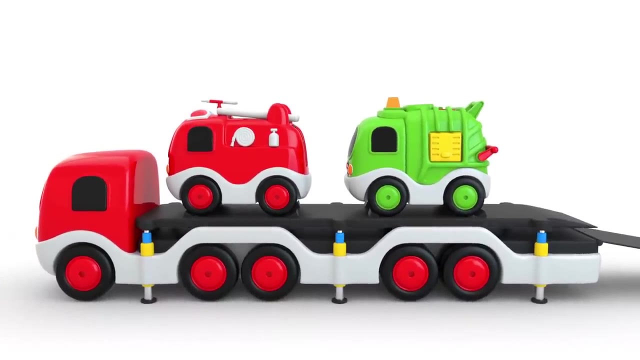 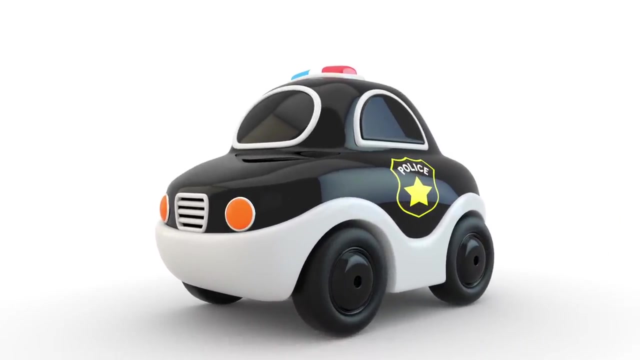 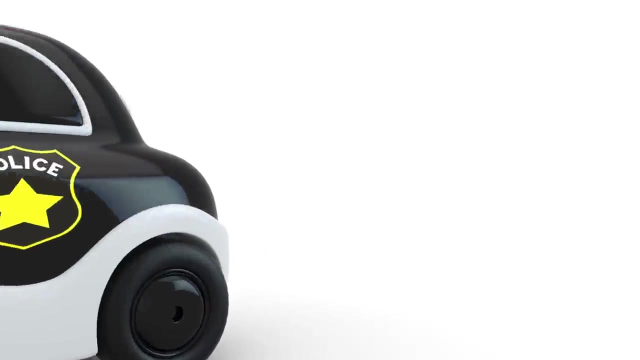 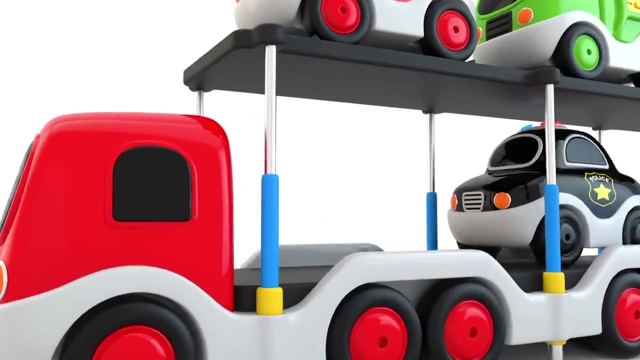 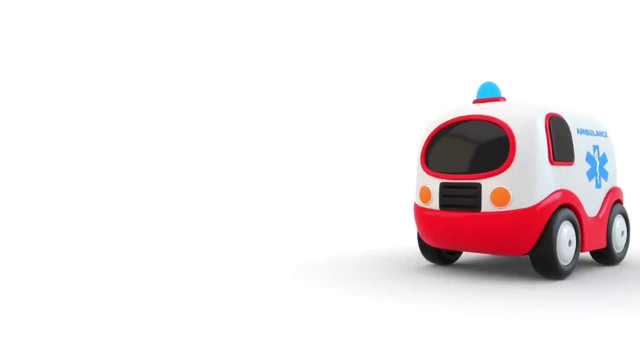 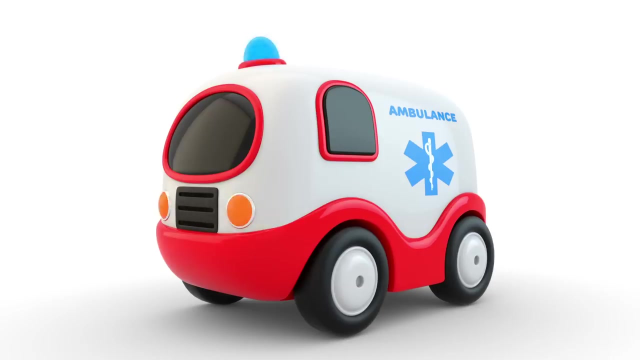 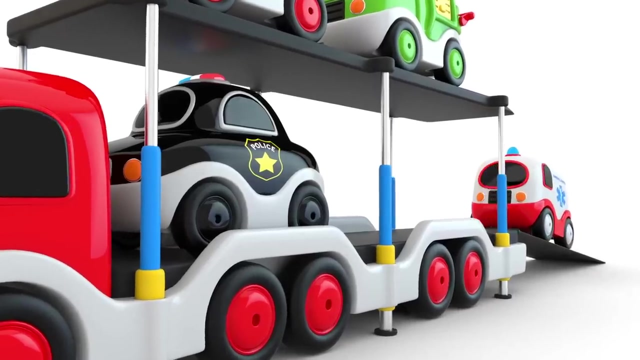 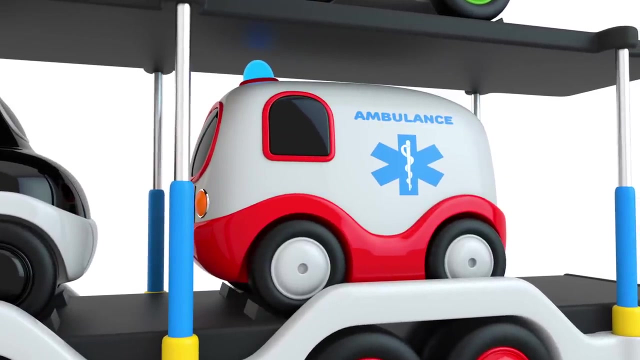 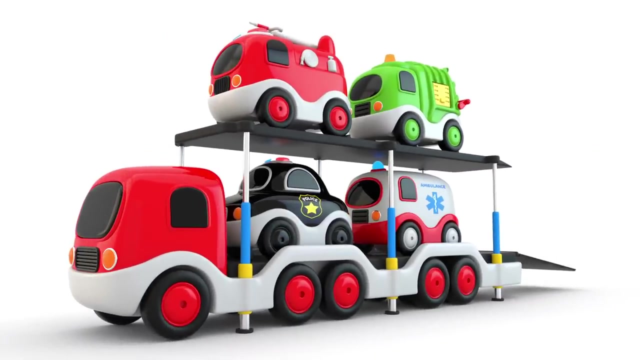 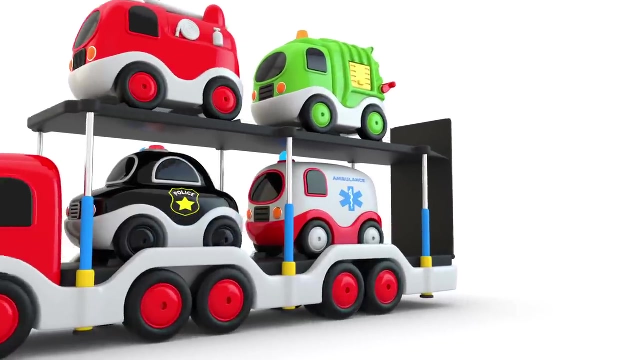 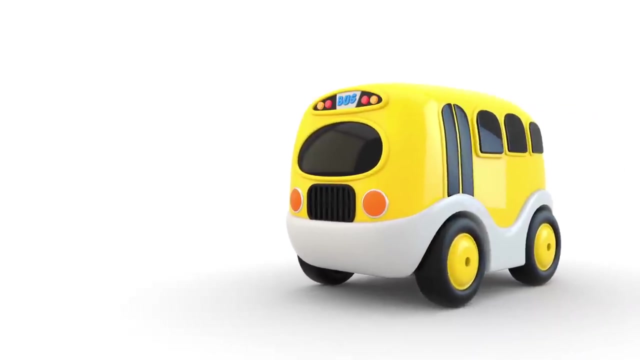 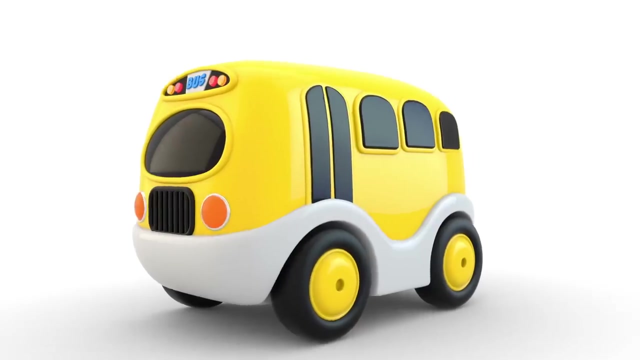 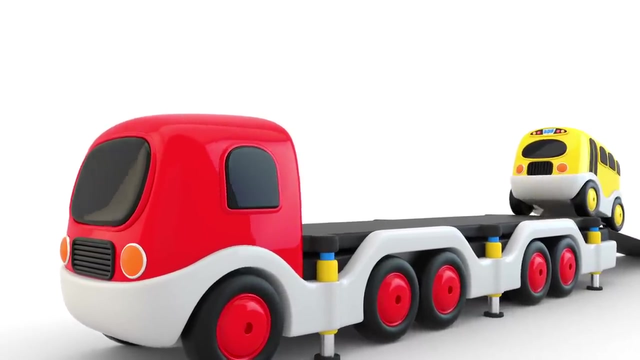 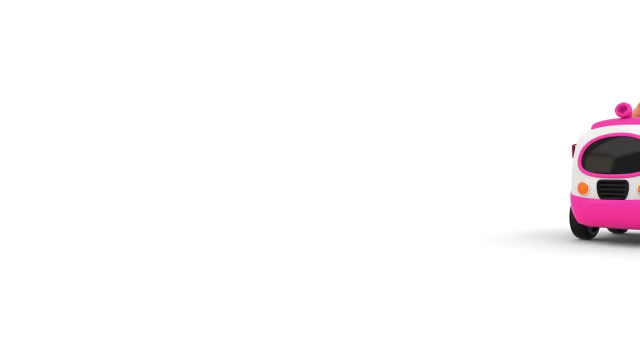 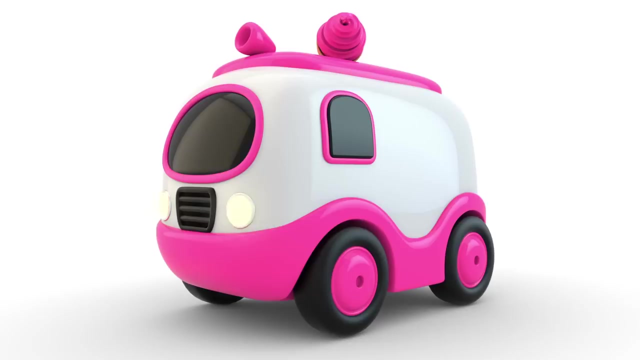 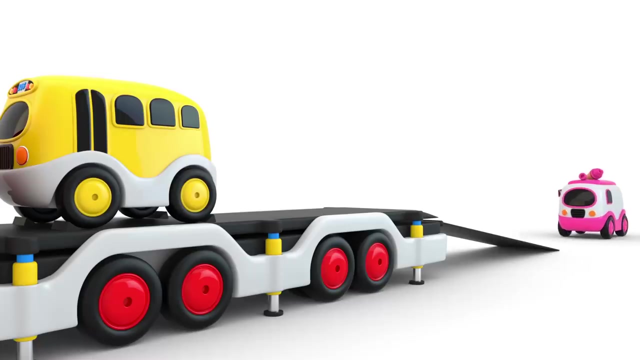 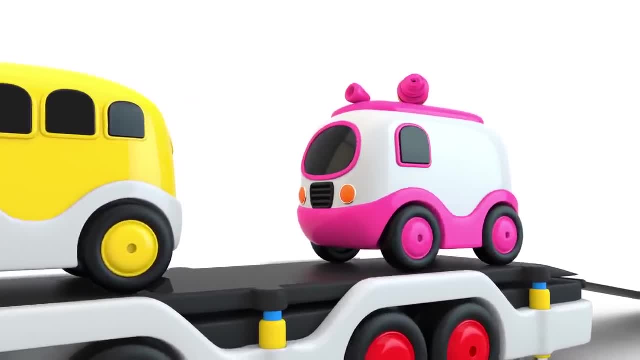 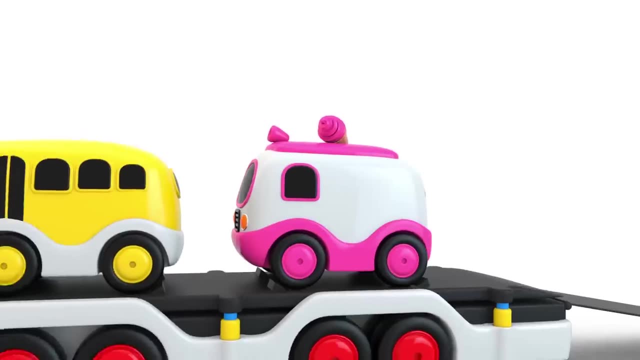 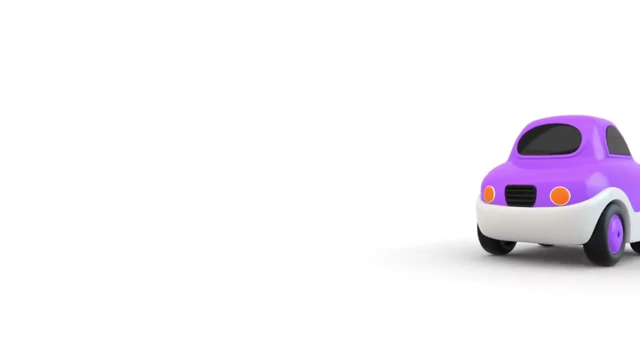 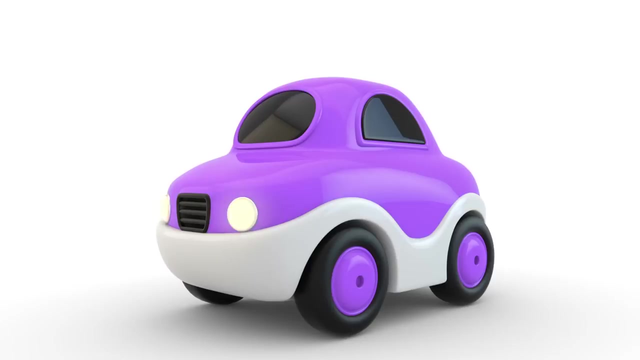 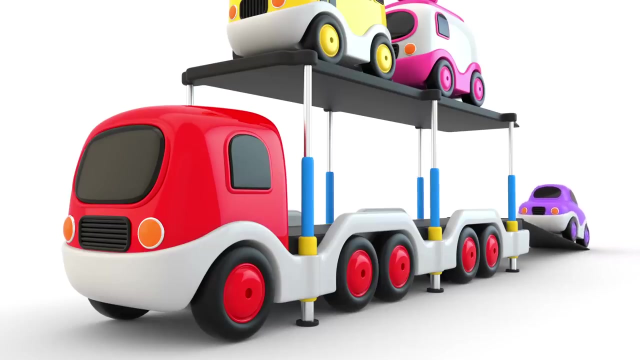 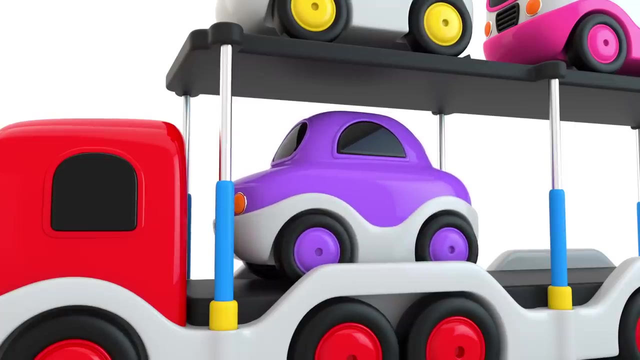 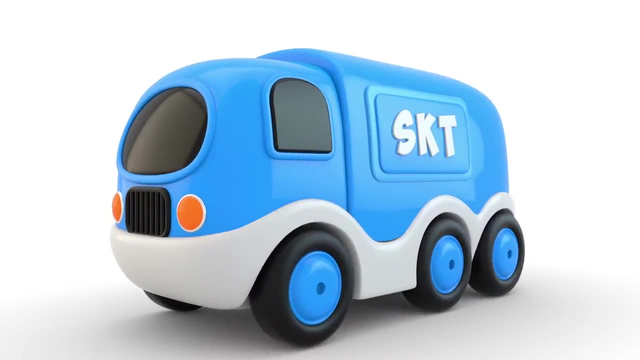 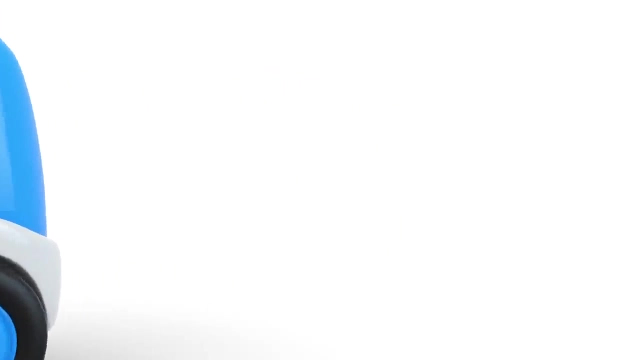 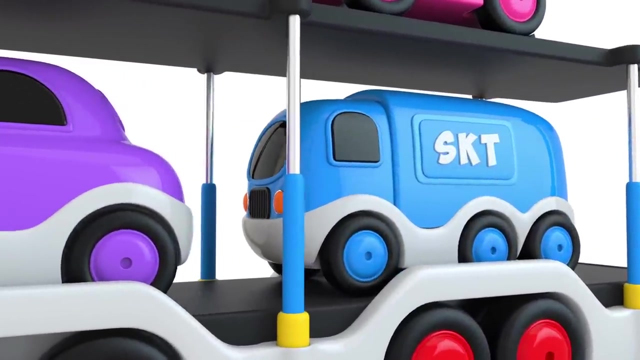 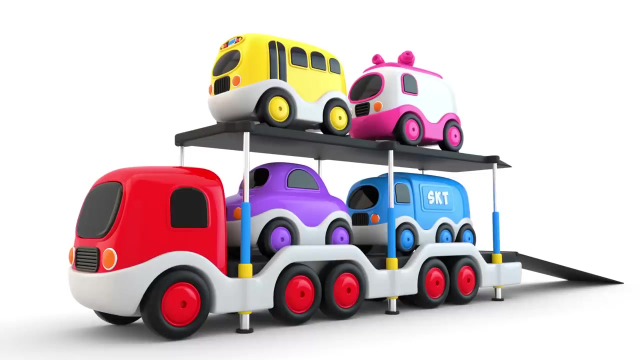 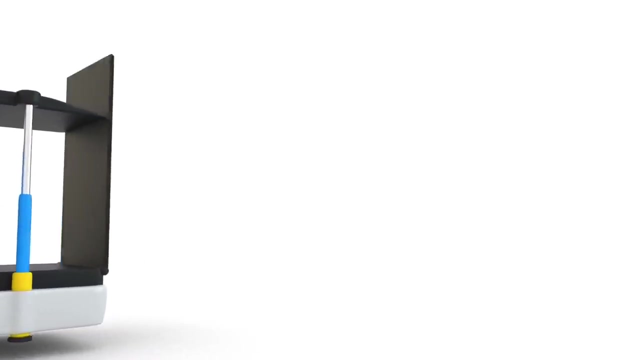 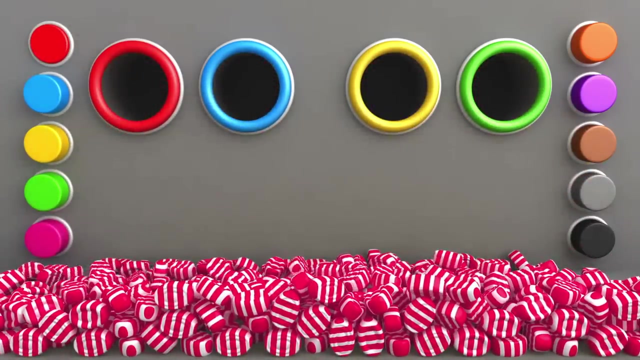 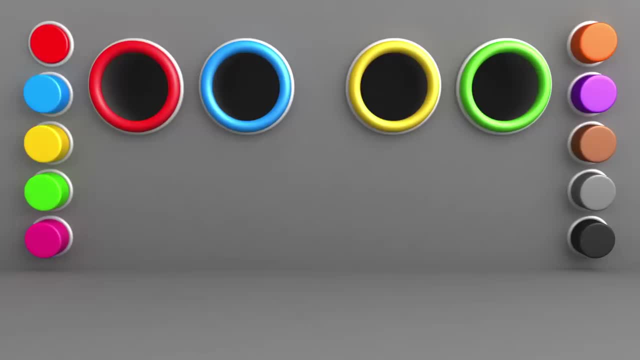 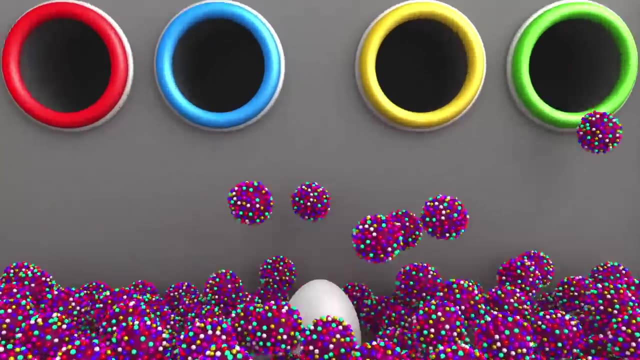 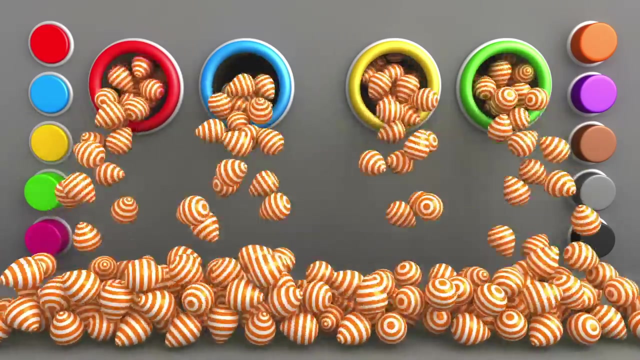 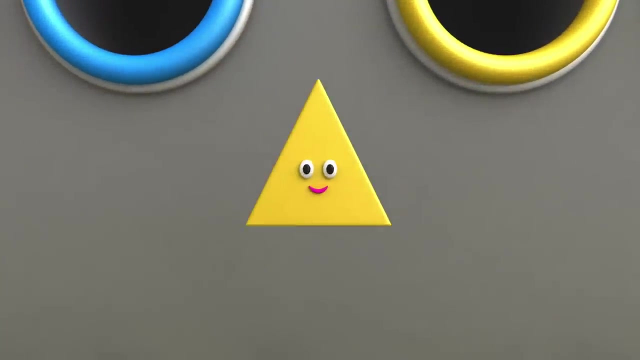 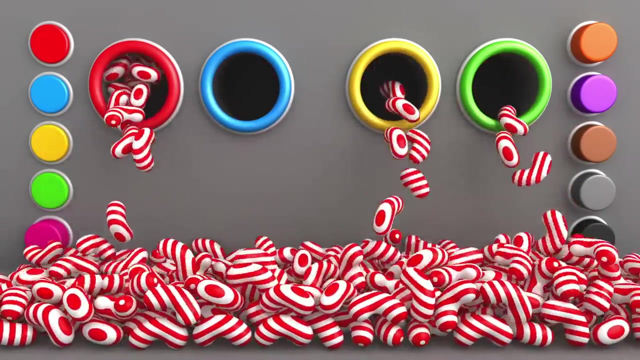 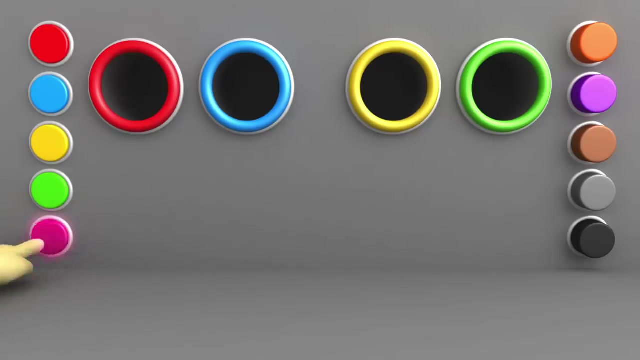 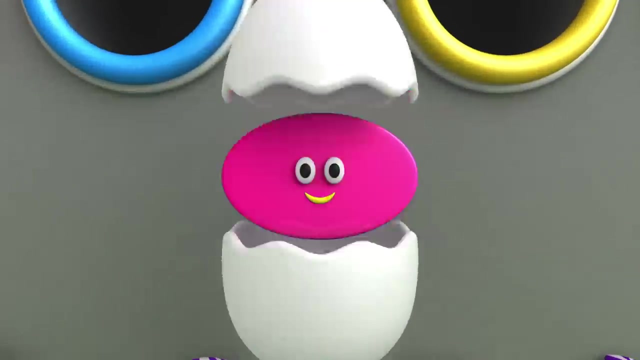 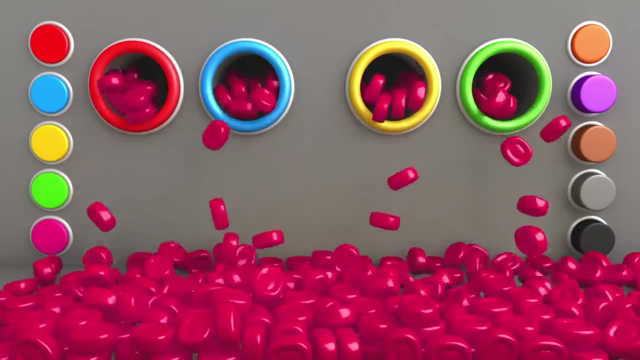 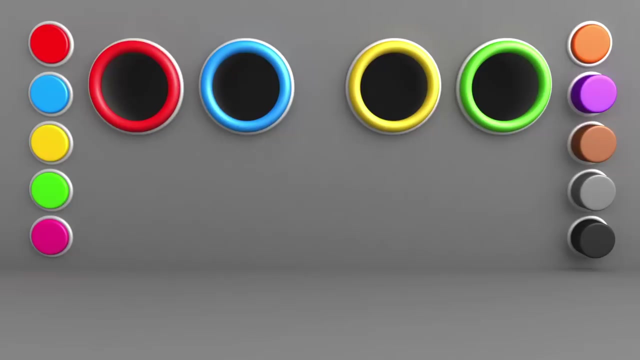 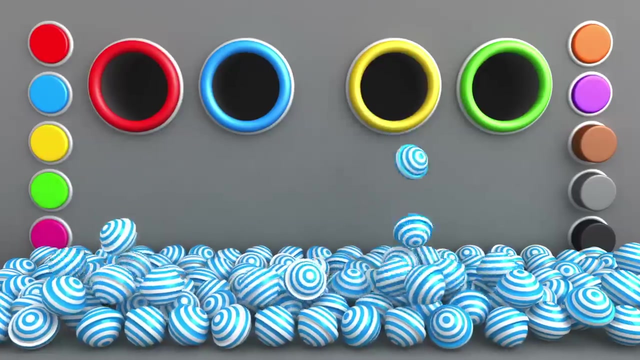 Surprise Circle, Wow Yes. Surprise Square: Wow Yes. Surprise Triangle: Wow Yes. Surprise Rectangle: Wow Yes. Surprise Oval: Wow Yes, Yes. Surprise Cross: Wow Yes, Yes.